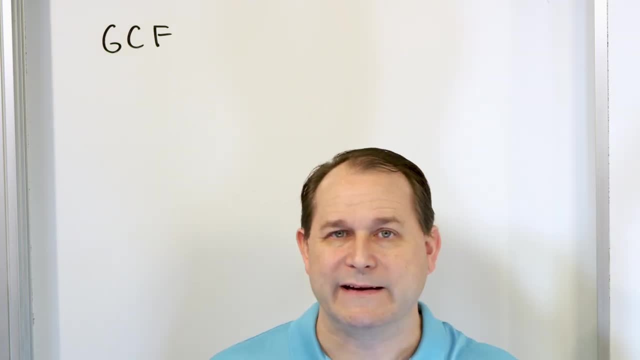 and all we have to do is pick the biggest number that's in the same in both lists. That's all. it is The greatest factor that is common to both. That's what we're doing: Greatest common factor. Now, the first thing you need to know is: what is a factor? anyway, When you hear the word factor in 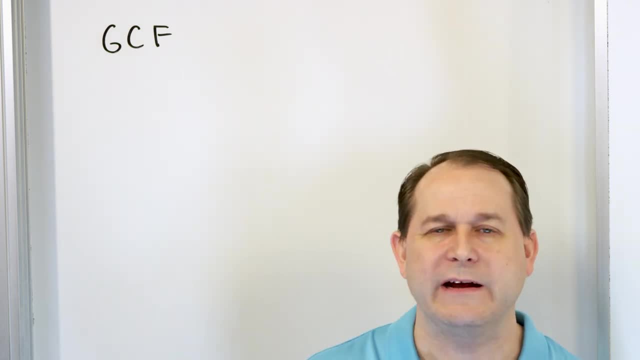 math. this is what I want you to think about. A factor is just a number. It's a number, that's just the numbers that multiply together to give you the number that you want that you're talking about. I'll say that one more time: The factors of a number are all of the numbers that could be. 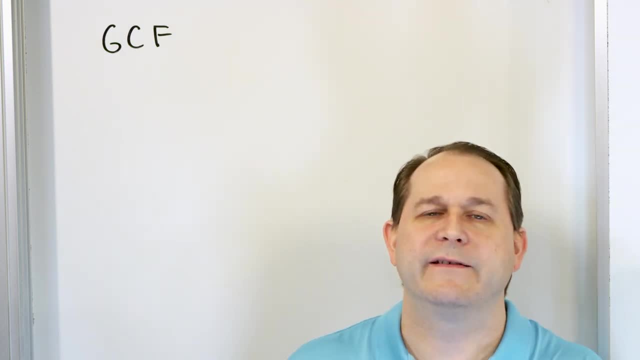 multiplied together to give you the number you care about. So, for instance, the number 10,. right, You know that 1 times 10 is 10.. So 1 and 10 are factors, because they can be multiplied together to give us 10.. 2 and 5 are also factors of 10.. Why? Because 2 times 5 is 10.. So when we 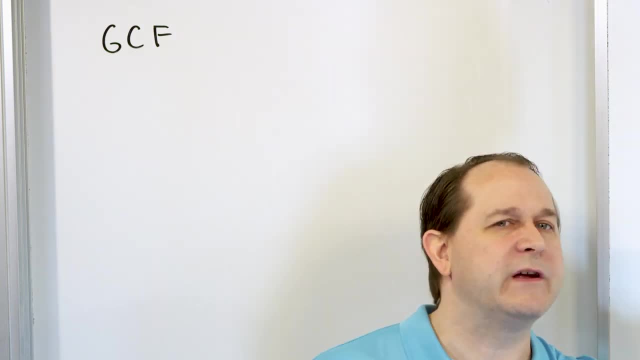 say factors of numbers. all we want to figure out is what are all of the numbers that could be multiplied to give us the number that we care about, which in this case, the example was 10.. But we can do it for any number that we want. All right, So let's talk about the greatest common. 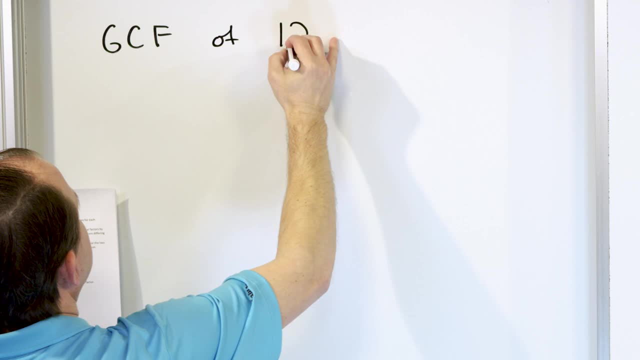 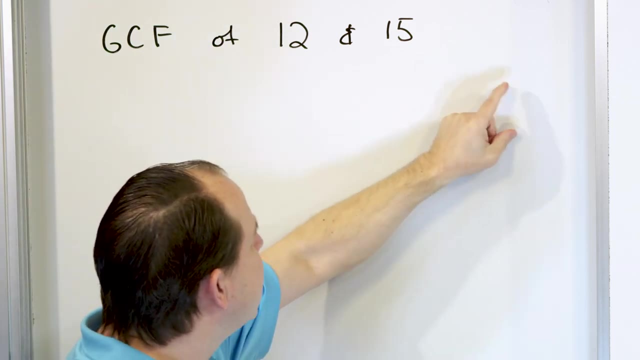 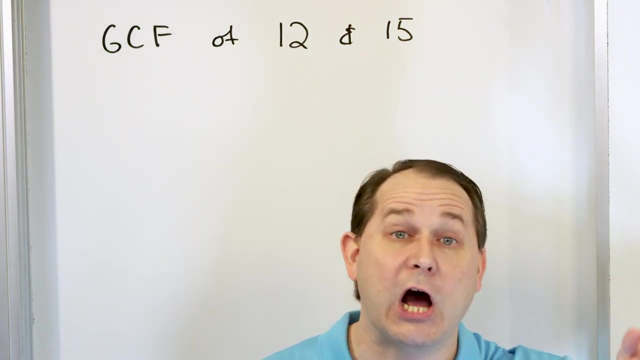 factor of the number 12 and the number 15.. So what we have to do is find the factors of 12 and write them down, and find the factors of 15 and write them down, And then, once we have all of the list of factors, we just pick the biggest one that is common in both lists. So let's write that. 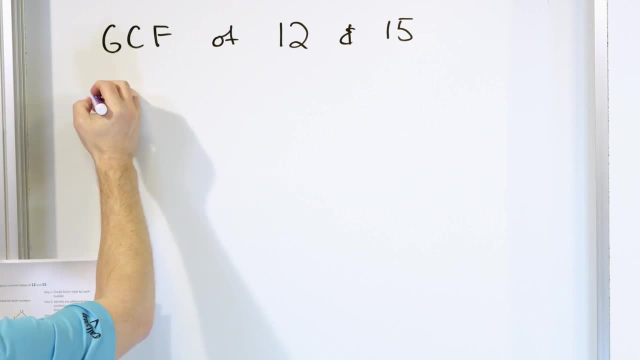 down Greatest common factor of 12.. So what we say is we write down these are the factors, If I can write the word factor, factor of 12. And underneath it we're going to write the factors of 15.. And 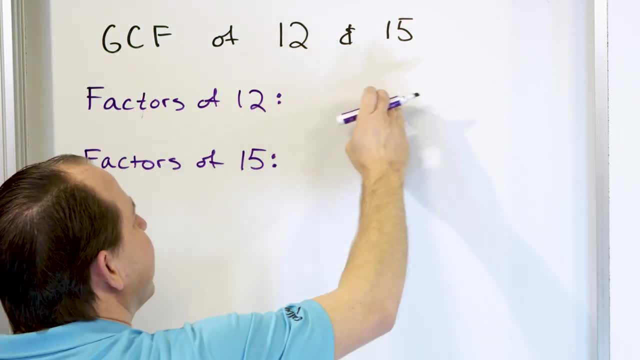 we're going to write these list of factors down And then, once we have the list, we'll just pick the greatest one that's common, And then, once we have the list of factors, we'll just pick the greatest one that's common to both lists, And that thing is going to be what we call the greatest. 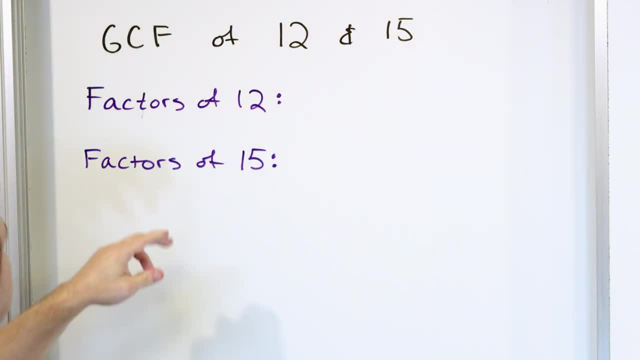 common factor. All right. So, in order to figure out, there's two ways to really think about it. The factors of 12. You need to think about what could be multiplied together to give you 12.. Another way of thinking about it is: can the number that you're considering be divided in? 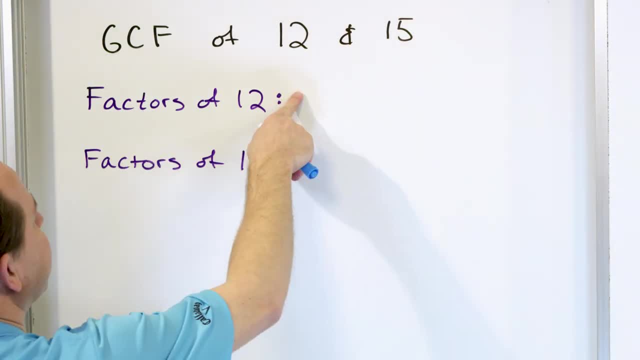 to 12 evenly. So let's talk about this. What about the number 1?? We're just going to go in order, starting with the number 1.. Can the number 1 be multiplied by something to give us 12? Well, 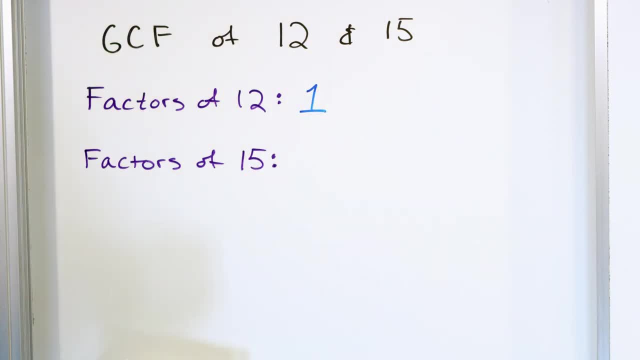 1 times 12 is 12.. So 1 is a factor. What about the number 2?? 2 times something gives me 12.. Yes, 2 times 6 is 12.. So 2 is a factor. All right, What about the number 3?? Well, 3 times 4 is 12.. So 3 is also a factor. So, 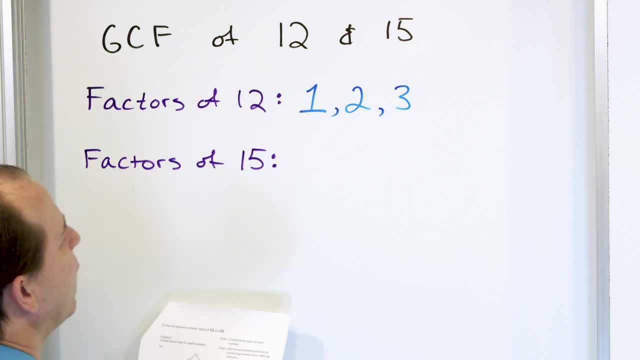 it's starting to look like every single number is a factor. That's not really quite right, but let's keep going. What about 4?? 4 times something can give me 12.. Yes, 4 times 3 is 12.. 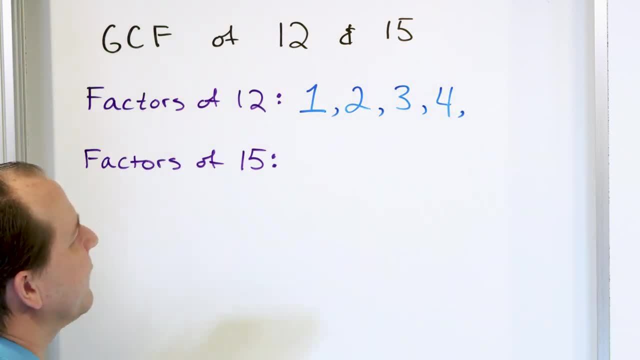 So 4 has to be there. Now, here we've come up against the number 5.. 5 is a factor of 12.. 5 times what is 12?? Well, there is nothing that 5 can be multiplied by to. 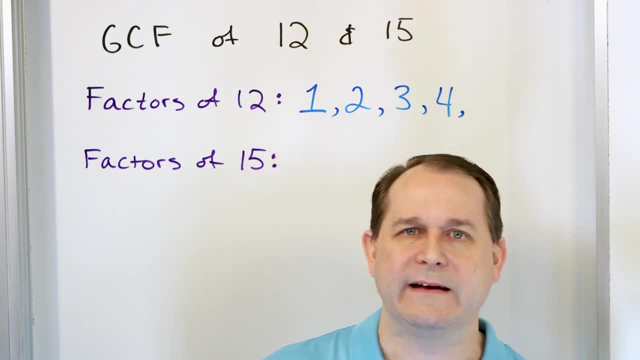 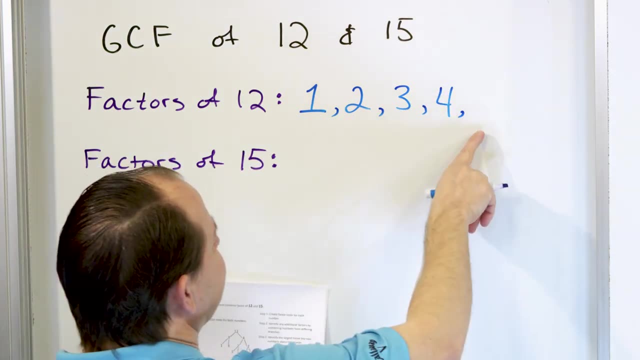 give you 12.. So it's not a factor. You see, only things that can go into the factor list are the things that can be multiplied to give you 12.. So let's skip over 5.. What about 6?? Well, 6 times 2. 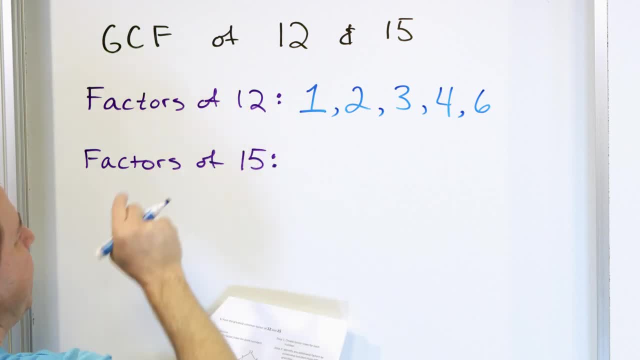 is 12.. So 6 is a factor. What about 7?? No, 7 can't be multiplied to give me 12.. What about 8?? No, 8 times 2 is 16.. It doesn't give me 12.. What about 9?? No, 9 is not a factor. 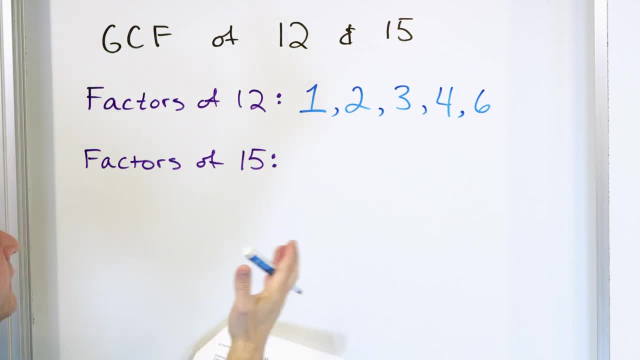 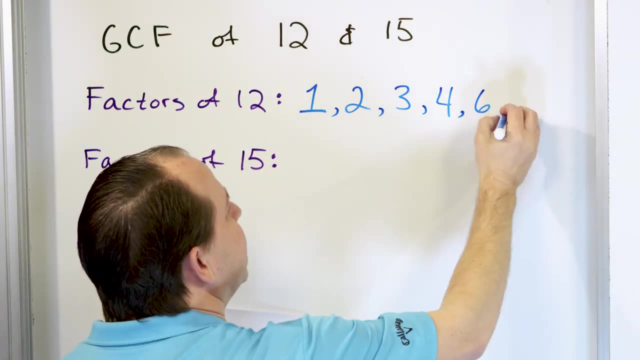 10. 10 is not a factor. 11. 11 is not a factor. I can't multiply them to give me 12.. But when I get to the number 12 itself, 12 times 1 is 12.. So actually 12 is also a factor. 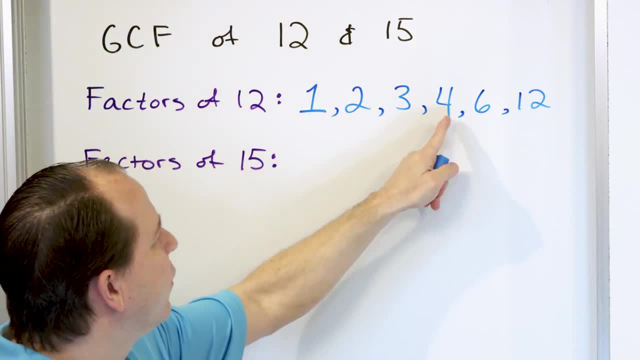 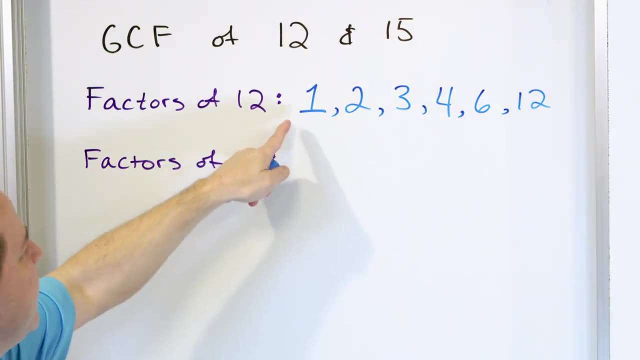 All right. So the factors of the number 12 are 1,, 2,, 3,, 4,, 6, and 12, because every one of those numbers can be multiplied by something to give me 12.. Another way of thinking about it is that: 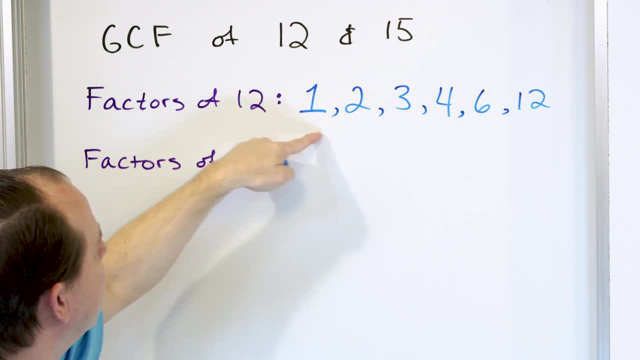 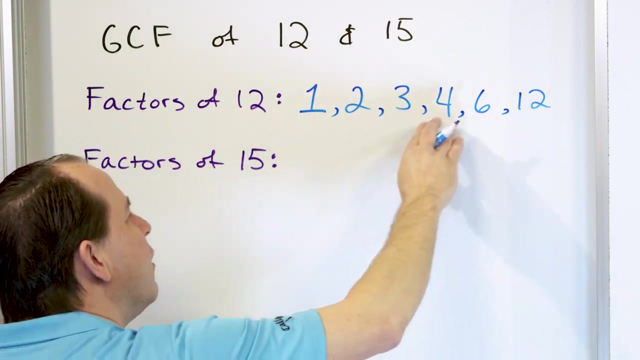 all of these numbers can be divided in evenly into 12.. 1, that goes in a whole number of times 12 divided by 2 would be 6.. It goes a whole number of times 12 divided by 3,, 12 divided by 4, 12 divided by 6, 12 divided by 12.. They all go a. 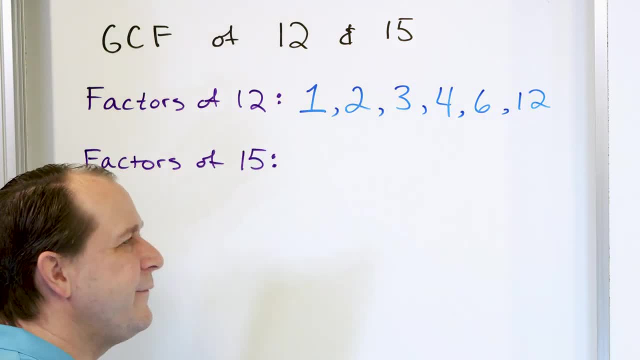 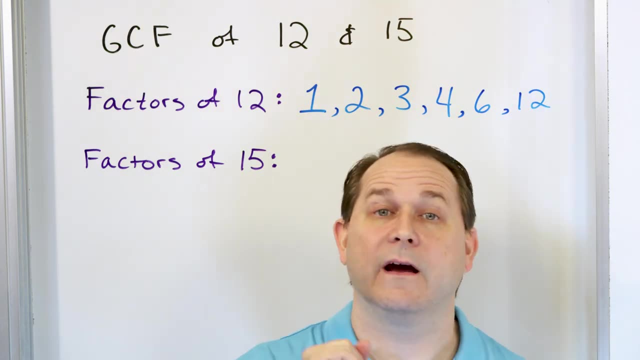 whole number of times, So they're all factors. So you can think of factors as being they can be multiplied together to give us a number. Or you can think of factors as being able to be divided in a whole number of times perfectly, And those are also called the factors. Now we have to do. 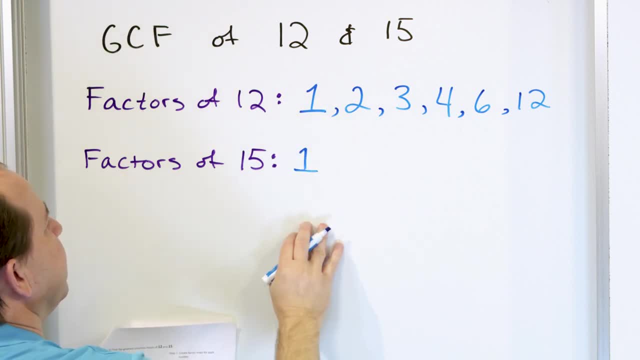 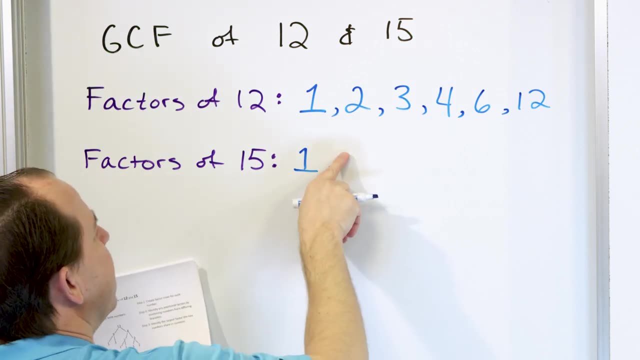 the process for the number 15.. Well, 1 times 15 is 15, so that's a factor. 2, is 2 a factor? No, because 2 can't be multiplied by anything, to give me 15.. What about 3?? 3 times 5 is 15,. 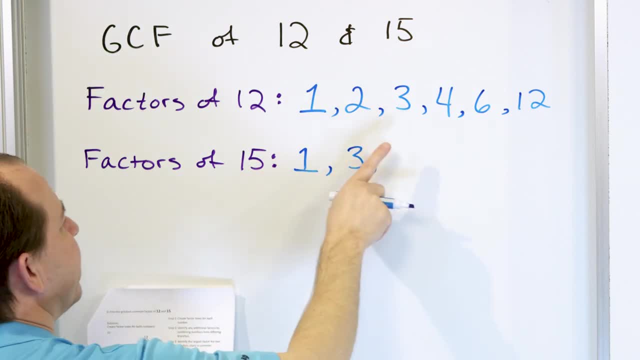 so that goes in. What about 4?? 4 is not a factor. What about 5?? 5 times 3 is 15, so 5 is a factor. What about 6?? Nope, 6 can't be multiplied to give me 15.. What about 7,, 8,, 9,? 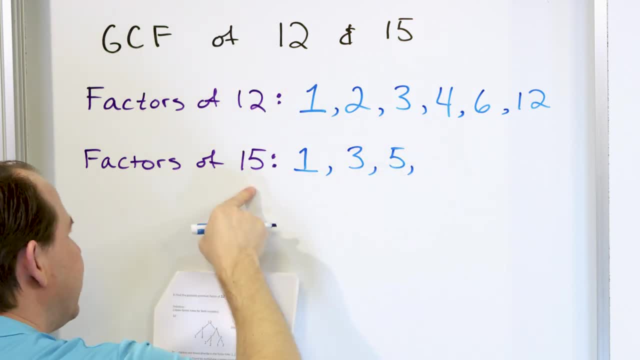 10?? Nope, none of those are factors. 11,, 12 can't be multiplied to give me this 13,, 14,. the only other factor is the number 15, because 15 times 1 is 15.. So another way of. 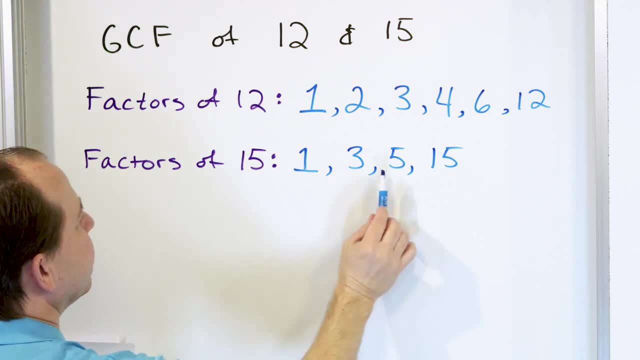 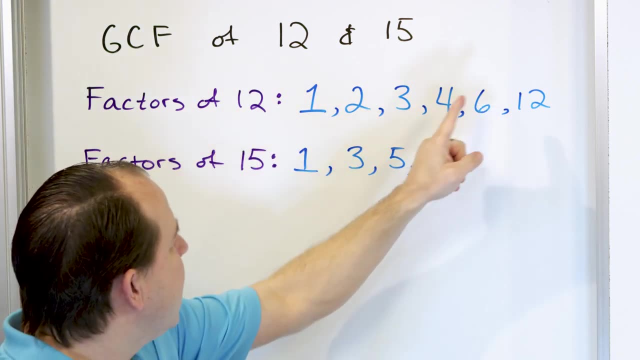 thinking about it is: 1 can divide into here, 3 can divide into here, 5 can divide into here, 15 can divide into here, but no other numbers can. So here are the factors of 12, and here are the. 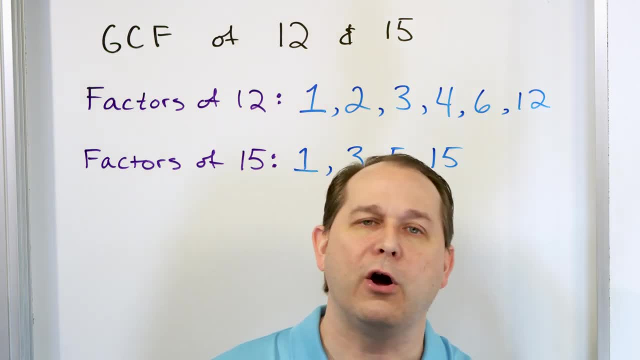 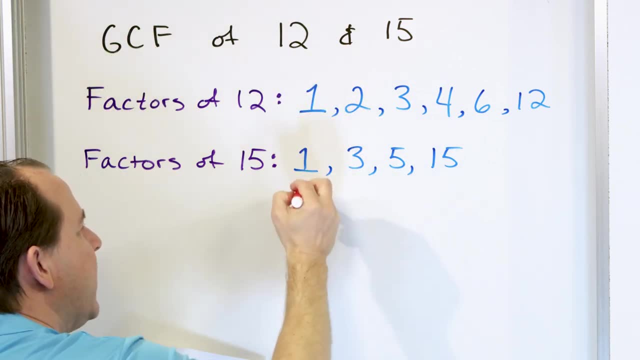 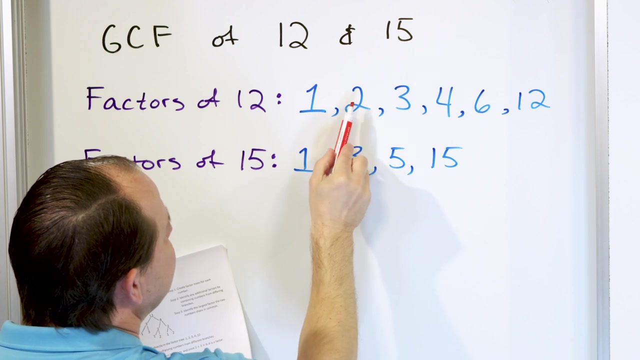 factors of 15.. And we have all of the factors written for both. All we have to do now is just look in the list and figure out what is the greatest common factor. Well, 1 is a common factor, but it is not the greatest common factor because we have to continue looking. 2 is in this. 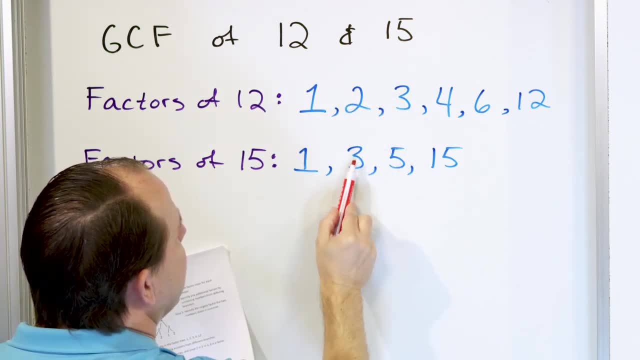 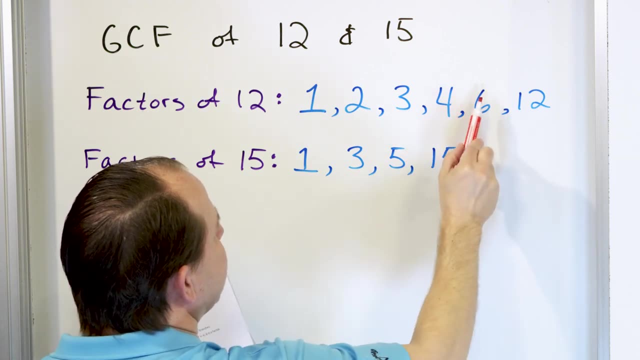 list, but 2 is not here. 3 is in both. Then we have 5 here, but 5 is not over here. 4 is here, but 4 is not over here. 15 is here, but it's not here. There's no other commonality, Only 1 is. 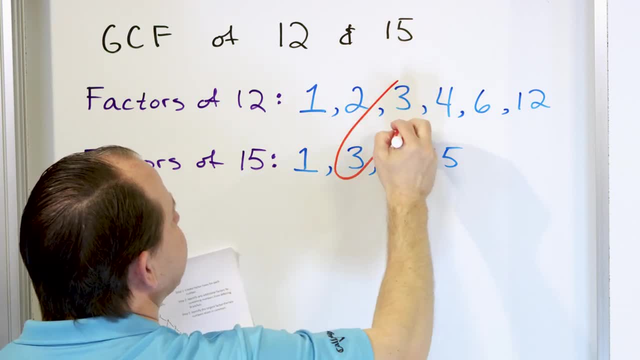 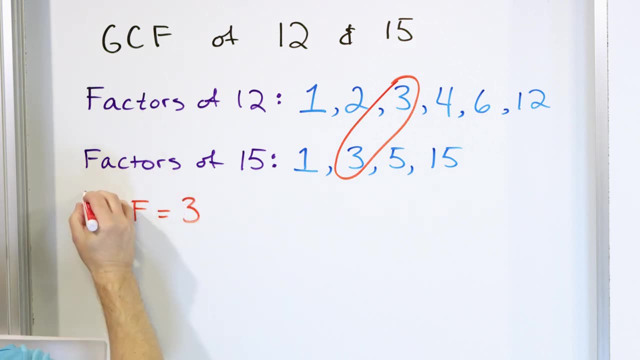 common and 3 is common And 3 is the greatest common factor. It's the largest factor, So the greatest common factor is 3.. I know that this process seems cumbersome and hard and weird, but after a while you're going to get very good at writing the factors down. 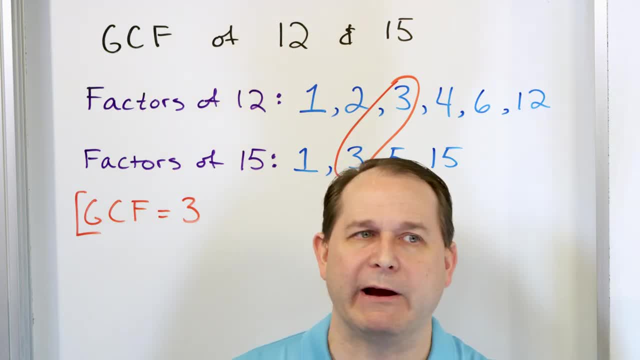 and then you're going to be very good at figuring out the largest one That's common. That's all you're doing, All right, a couple things I want to say before we move on to the next problem. Notice that for the factors of 12, we had to go through and figure out all the factors. 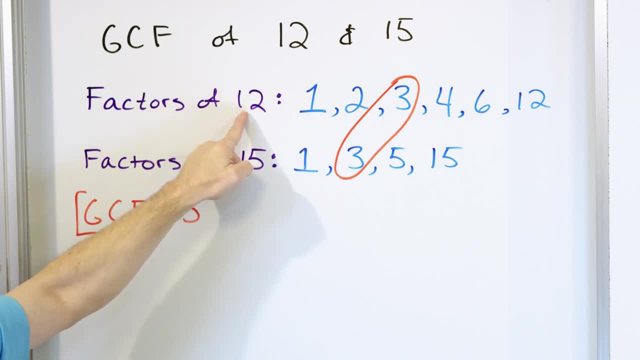 but notice, the number 1 is a factor and the number itself, 12, is always a factor. The reason number 1 and the number itself, 12 in that case is a factor is because 1 times 12 is 12.. Notice, over here, 1 was a factor of 15, and 15 was also a factor of 15.. So the number 1 and 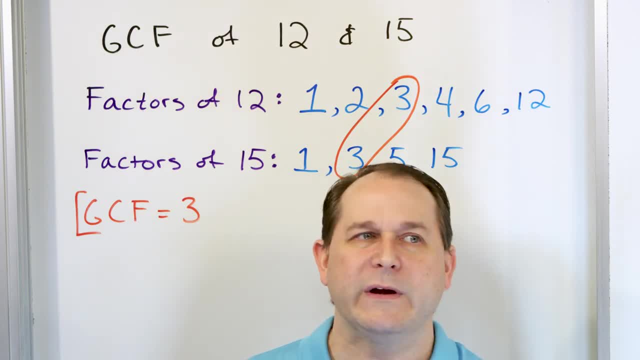 the number itself are always factors of the number. So really the list. we have a big list here, but really the number 1 and the number itself is always a factor. The number 1 and the number itself is always a factor. All we have to do is find the other ones that are in the middle. 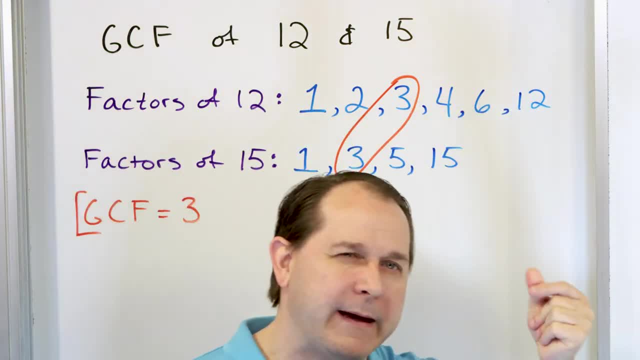 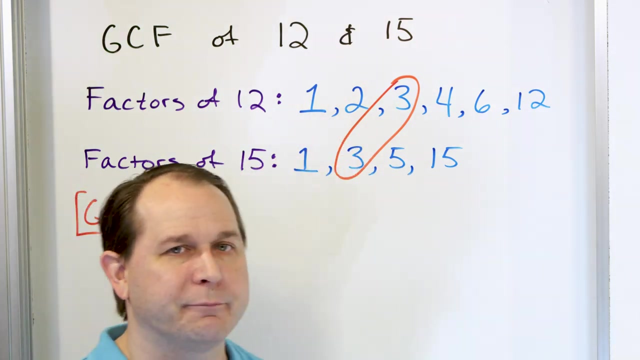 We could just go through this and find them all by thinking about them, because these numbers were pretty small. but if I ask you the GCF of a large number, it might be tough to find all the factors. So what I want to do is show you another way to find the factors that we didn't need it for this. 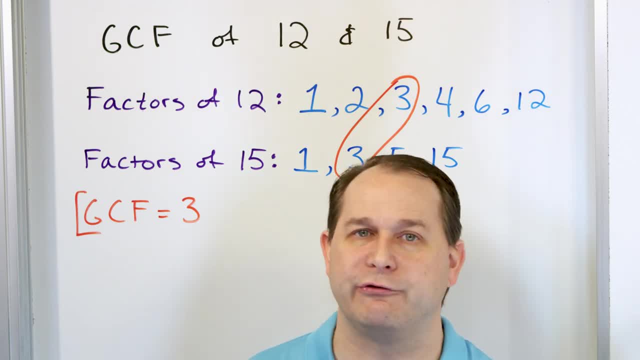 problem, but it's going to help us in a few problems when I give you larger numbers, So I'm going to show you for an easier problem, so you'll understand. It's actually kind of a fun process. What we're going to do is find what we call a factor tree. 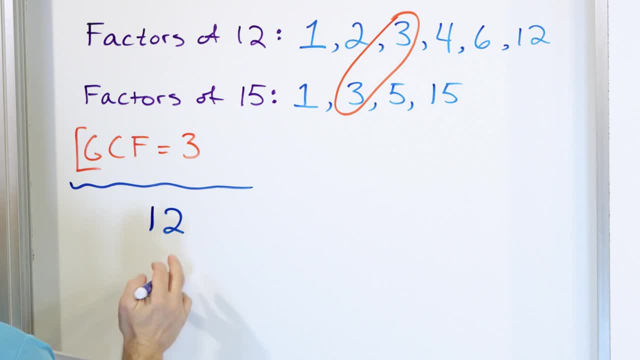 Let's say we want to find the factors of 12.. All you do is draw a little tree under here and think to yourself: what times, what can give me 12?? And you can pick anything you want. You can pick 2 times 6 to give you 12, or you can pick 3 times 4 to give you 12.. You have total freedom to do. 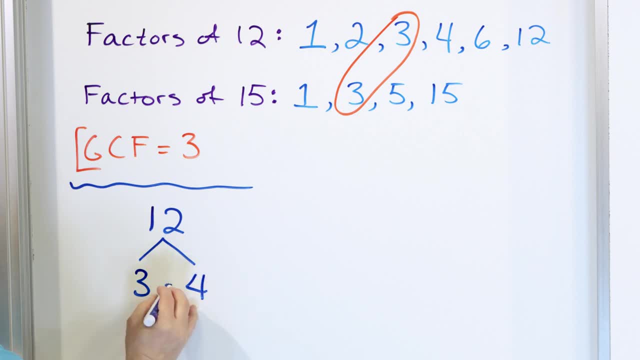 what you want. Let's pick 3 times 4 and put a little dot there. This is telling me that 3 times 4 is giving me 12.. Now over here under the 4, we try to split that up further. What times, what can? 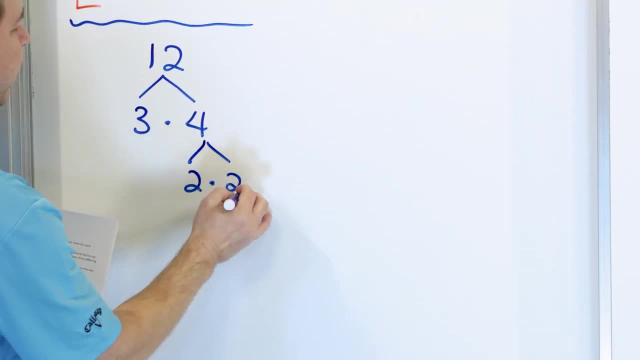 give me 4?? Well, 2 times 2 is the thing that I think of that can give me 4.. So what I've done is I've split the 12 into 3 times 4, and I've split the 4 into 2 times 2.. Now you can split the 3 into. 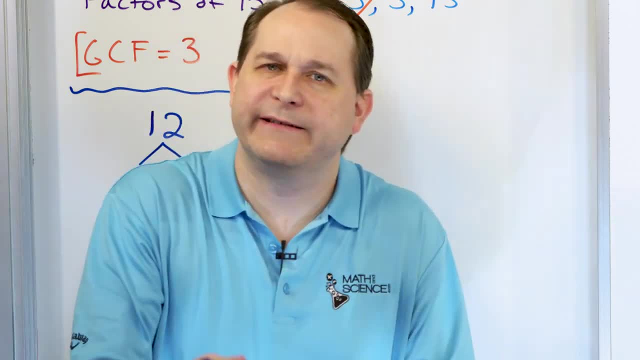 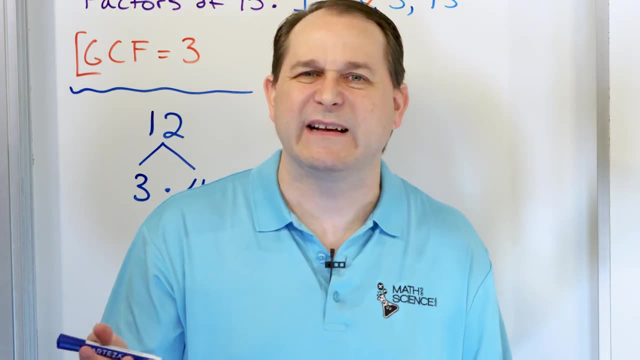 1 times 3, but notice that it doesn't really get any simpler because 1 times 3,- they're both simple- They're called prime numbers. We'll get into prime numbers later, but they basically can't be broken apart any further. 2 is also the simplest number you can get to. as well You can put 1 times. 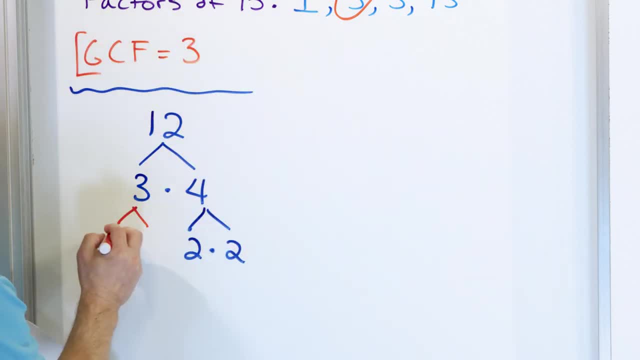 4. In fact I'll go ahead and do that in red. You could put like, for instance, 1 times 3,, but you can't go any farther because then you'll just keep breaking the 3 into 1 times 3, over and over again. 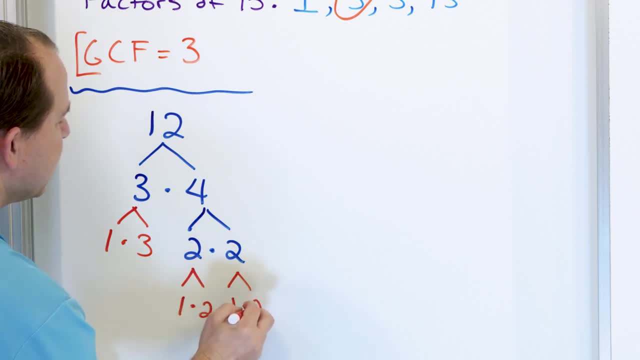 And you can make this 1 times 2, and you can make this 1 times 2,, but notice, you can't go any farther because you keep getting 2s, And so the tree is basically done here in blue, Now everything. 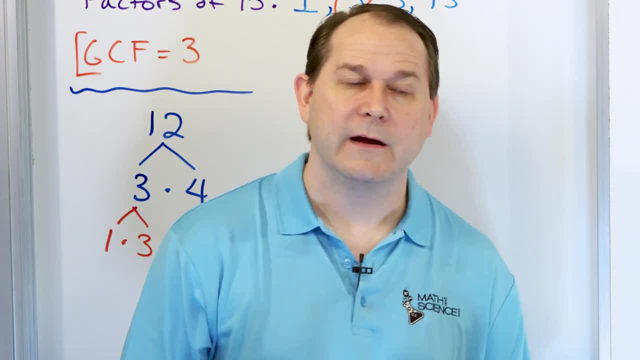 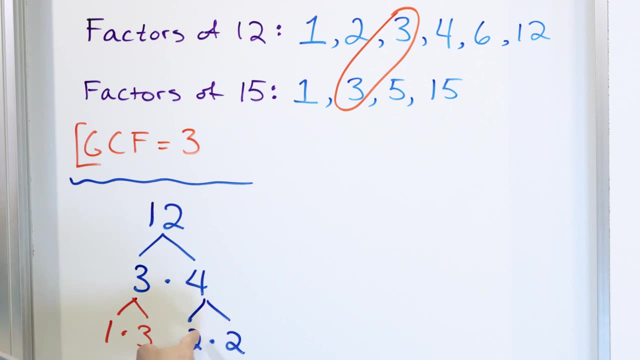 in this tree is a factor of the number 12.. Notice that the number 1 is here down here at the bottom. That's a factor of 12.. The number 2 is in this tree. Don't worry about the fact that it's in here a bunch of different times. You're just looking for. 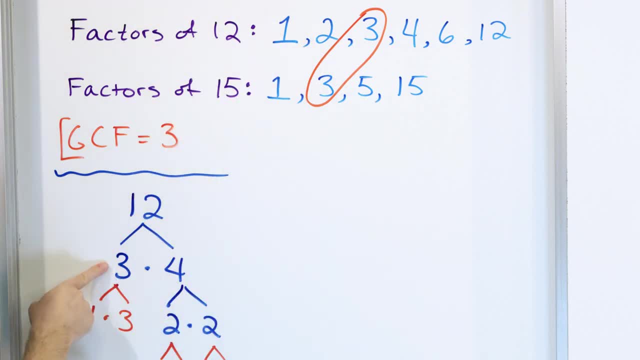 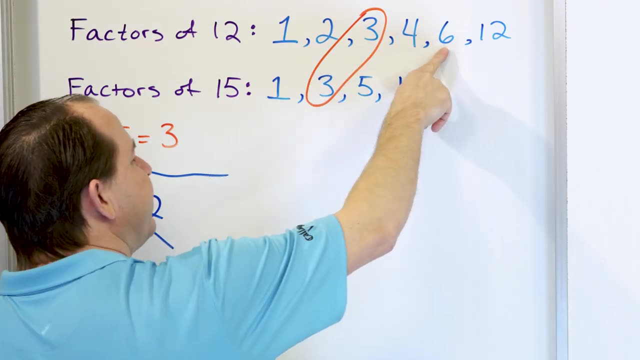 independent numbers. 2 is a factor here. 3 is in this tree. It is a factor here. 4 is in this tree. It is also a factor here. Now notice that we found that a factor was 6, but 6 is not in this tree. 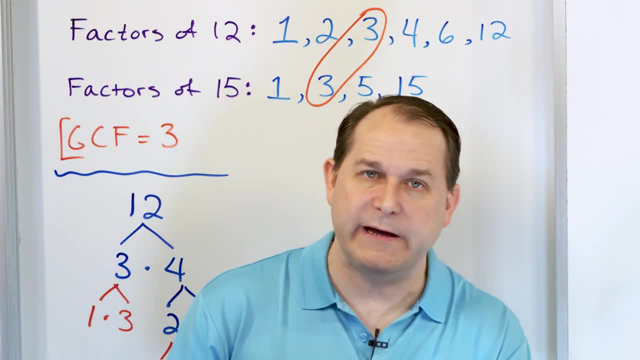 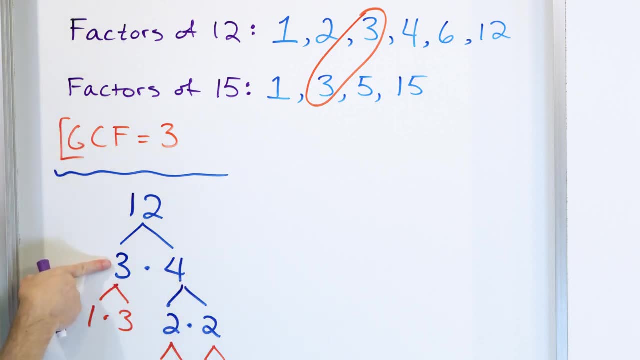 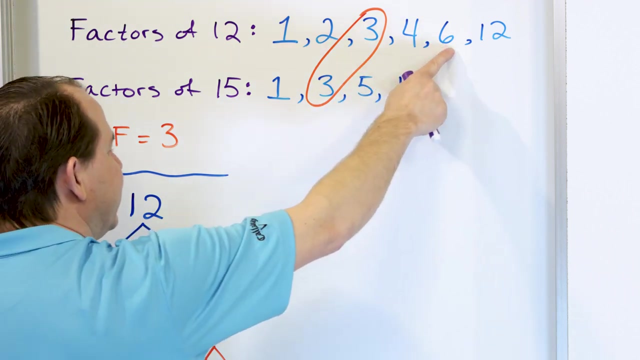 but that's okay, because the factors are going to be in the tree. or you can find factors by multiplying different branches of the number. So you see how you have a 3 here and you have a 2 here. Well, you can find more factors by multiplying 3 times 2 to give you 6, and that's why 6 is a. 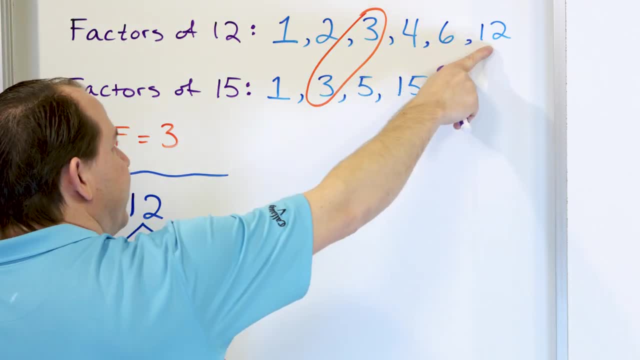 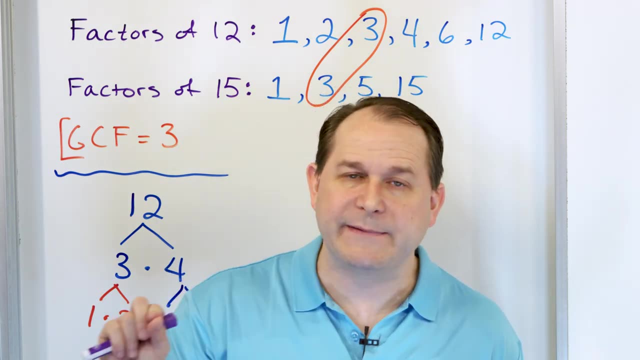 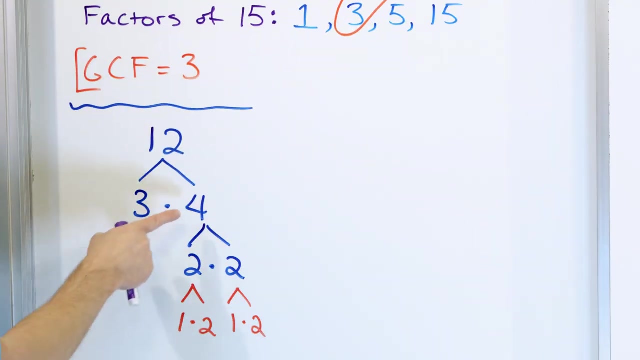 factor 4 times 3 is 12, and that's a factor here. And so basically, what you do is you build this tree. All of the numbers get pulled out of the tree, You write them down as your factors and any other numbers that pop up when you cross multiply branches of the tree. So 4 times 3 is 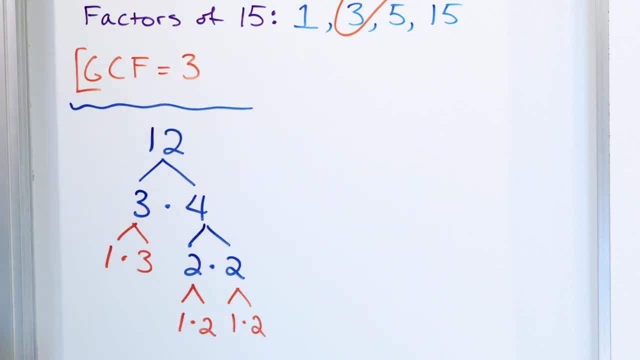 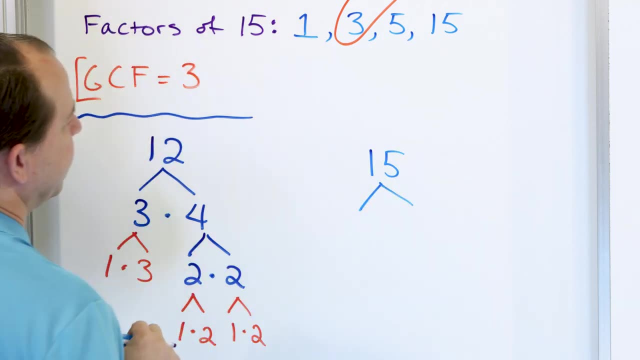 12. That's in there. 3 times 2 is 6.. There's no other numbers that you can come up with. Now let's do the same process for the number 15.. The number 15.. Well, the only thing I think of to. 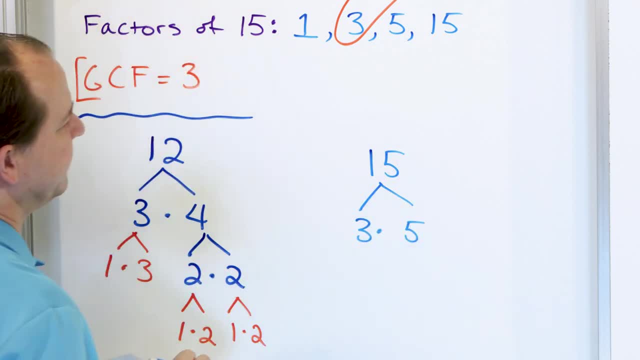 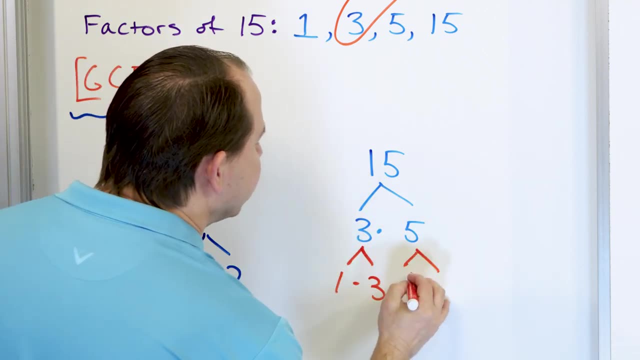 multiply, to give me: 15 is 3 times 5.. 3 times 5 is 15.. And then of course I can go down here and I can say: well, 3 is 1 times 3, and 5 is 1 times 5.. But you see how these don't get any. 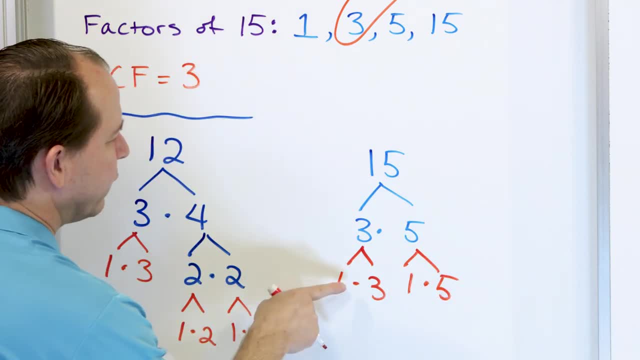 simpler, because the only thing that can multiply to give me 3 is 1 times 3.. The only time that can give me 5 is 1 times 5, and I can't do anything more than that because I keep getting 3,. 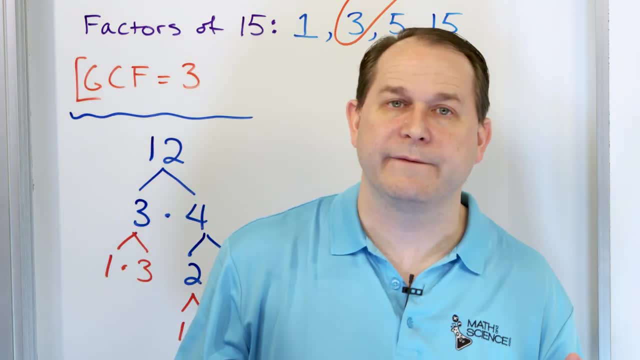 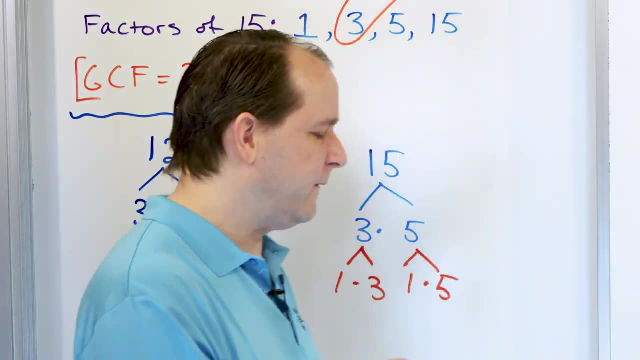 and 5.. These numbers here that can't be broken apart any further. they're called prime numbers because the only thing you can multiply to get 3 is 1 times 3, and you can't do anything more than that. So we look at this tree and we find our factors. We know that 1 is always a factor. 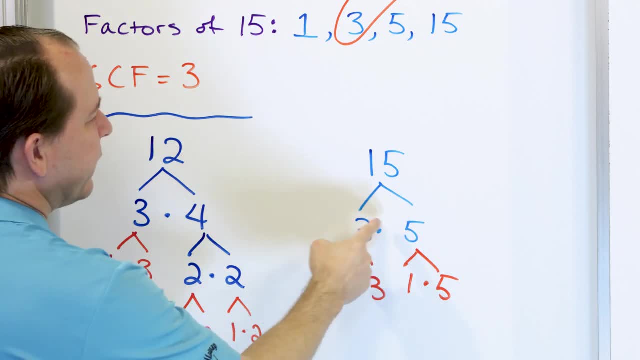 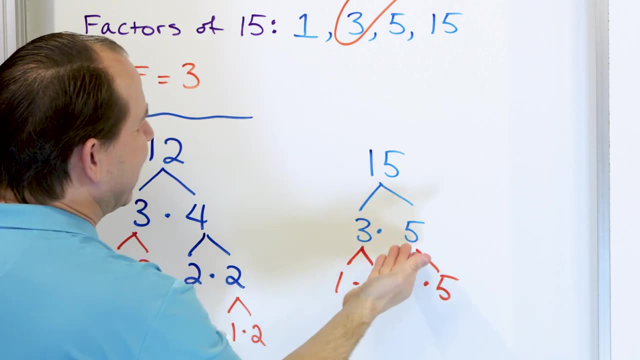 We know that the number itself, 15, is always a factor. The only other numbers in the tree are 3 and 5, so they're both factors, And then we can cross, multiply the branches 3 times 5,, but that's 15, and that's already in there anyway. 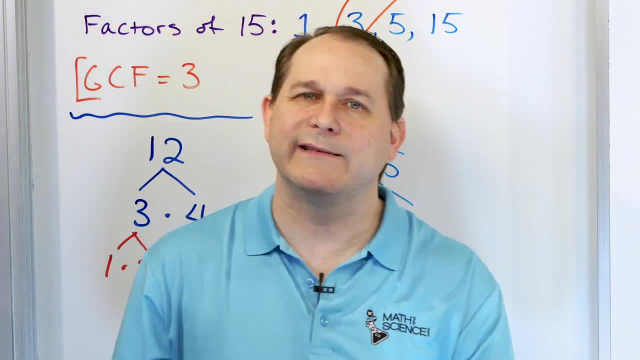 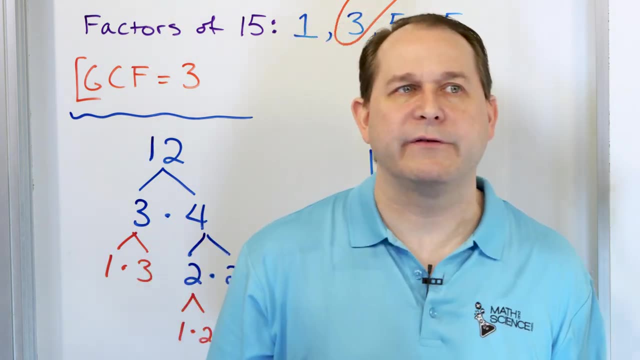 Problems. the numbers were really small, so the trees were not really necessary. You can just think through the factors like we did before. But when I give you, if I ask you tell me- the factors of 98 and 29,, then it's going to be really difficult to figure out all the factors. It's. 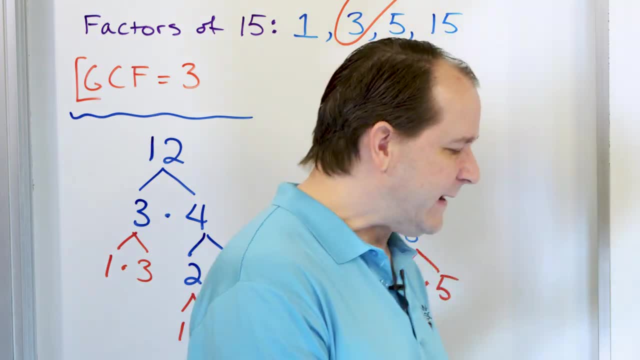 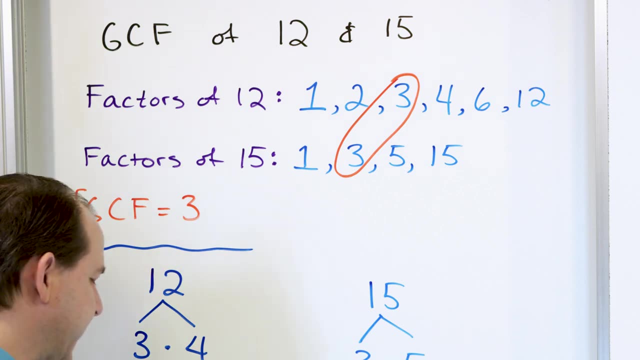 actually going to be way easier using a tree like this. So let's go ahead and move on to the next problem. The greatest common factor here was the number 3, and then we'll just kind of like learn this tree method here, kind of like on the back burner. 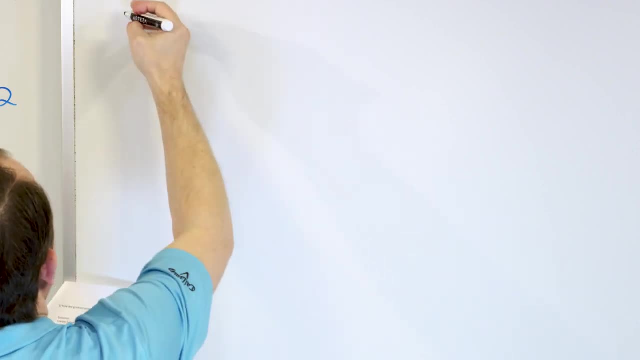 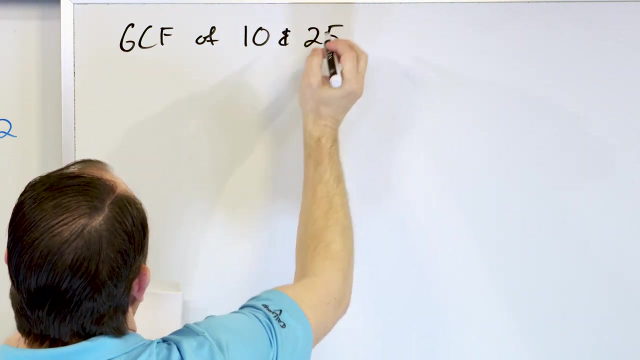 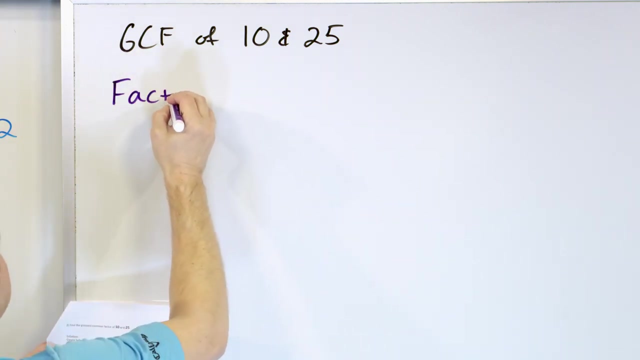 Bigger problems, it'll be more useful. Let's take a look at the GCF: GCF of 10 and 25.. 10 and 25.. So first we want to go through it kind of without using a tree, Let's use factors of 10.. 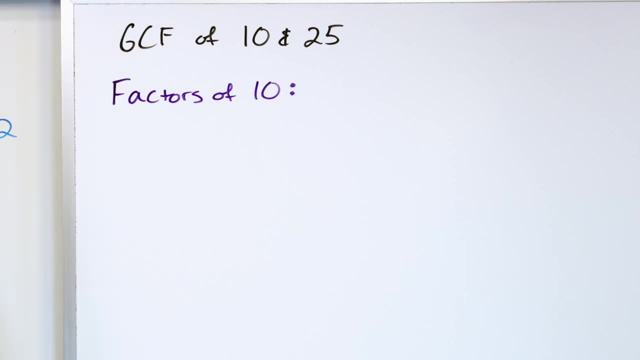 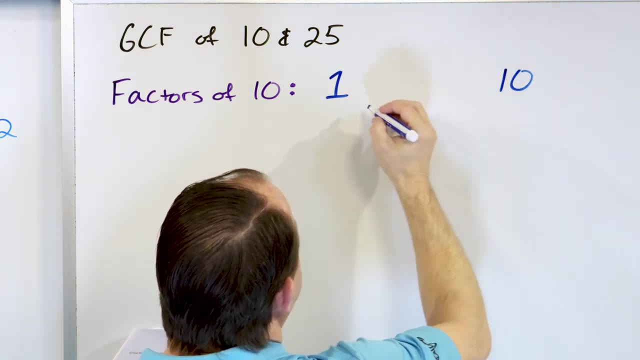 We want to figure out what can be multiplied together to give us 10.. We know that the number 1 and the number itself, 10, are always factors. So 1 and 10, are always factors. All we have to do is figure out what numbers are additional to that. What? 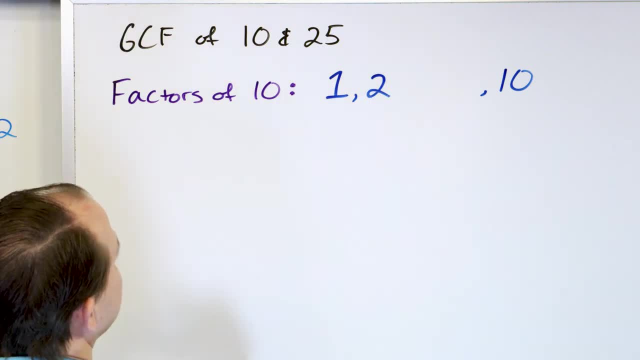 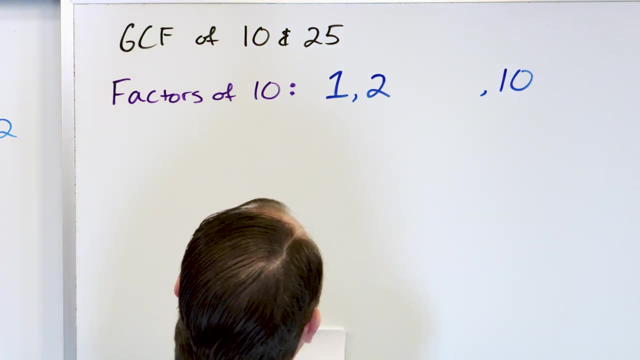 about 2?? Well, 2 times 5 is 10,, so that's a factor. 3, 3 is not a factor. 3 times 3 is 9, that doesn't work. 4 is not a factor, because 4 times 2 is 8.. What about 5?? Well, 5 times 2 is. 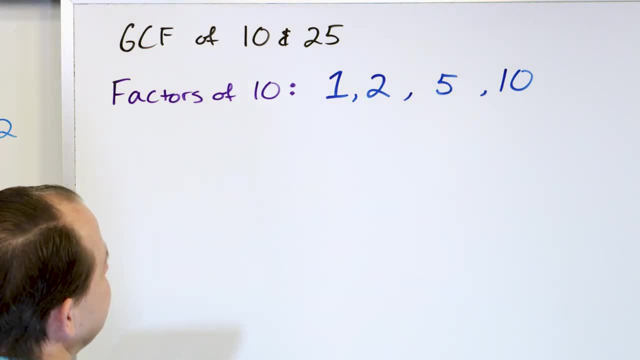 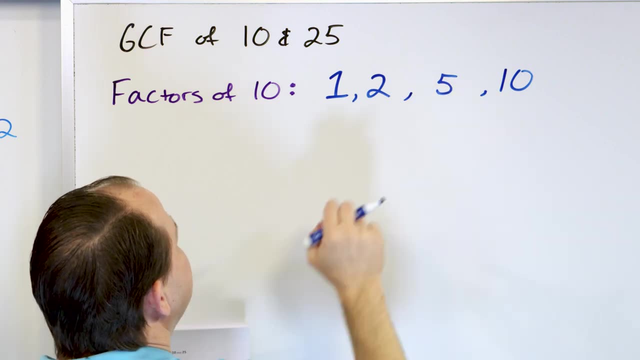 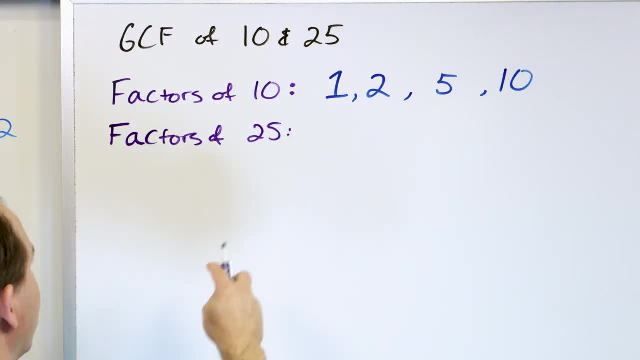 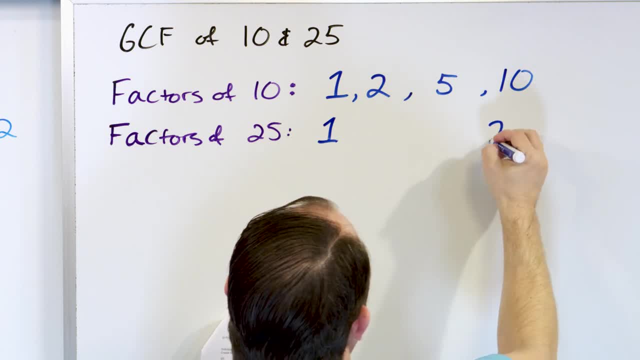 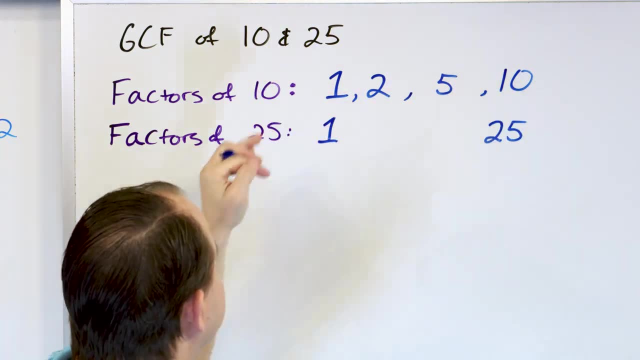 is also always a factor here, So I'll put- I'll just put it way over here- 25,. 25 is a factor, Because why 1 times 25 is 25, just like 1 times 10 is 10, so there are factors. 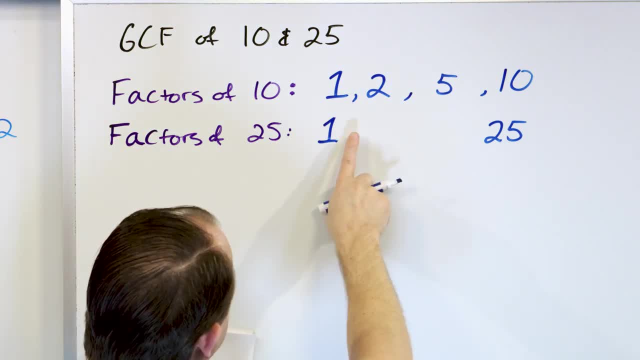 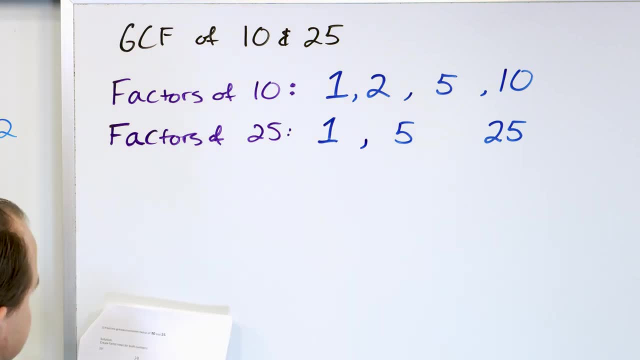 Alright, is 2 a factor? No 3? No, 4? No, But 5 is a factor, because 5 times 5 is 25, so I'll put 5 here. What about 6?, 7?? 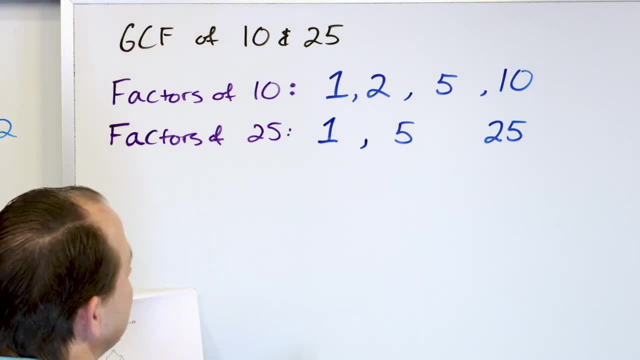 8? 8 times 3 is 24.. 9? 9 times 3 is 27.. 10? 10 times 3 is 30.. 10 times 2 is 20.. None of those are factors. 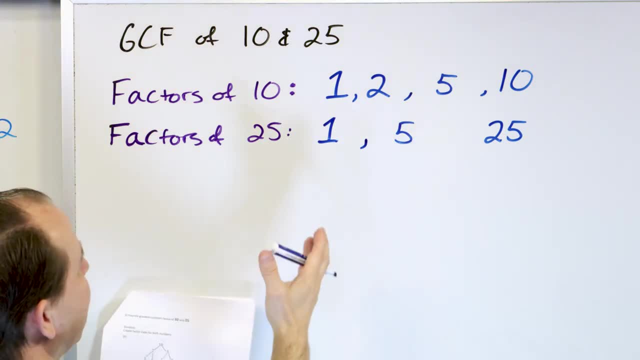 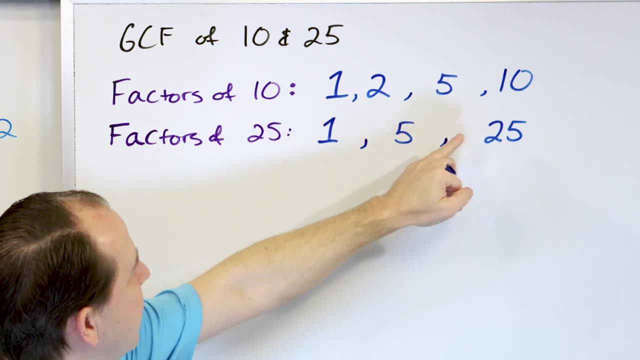 11,, 12,, 13,, 14,, 15,. none of those are factors because I can't multiply them by anything to give me 25.. So actually the number 25 only has 3 factors: 1, 5, and 25 itself. 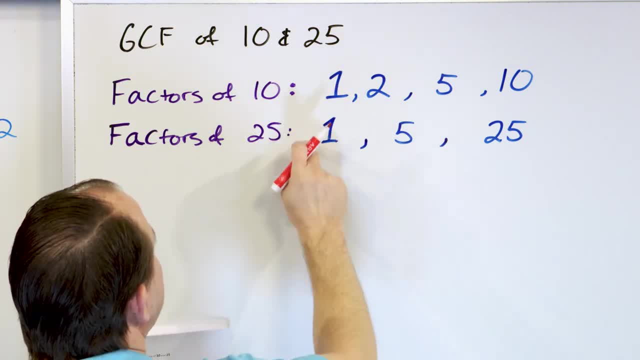 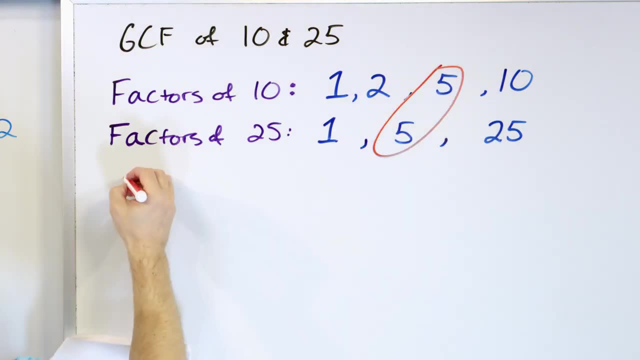 So the last step is to figure out what factors are common. 1 is a common factor, 5 is a common factor. Those are the only common factors and the bigger one is a 5.. So we say the GCF is equal to 5.. 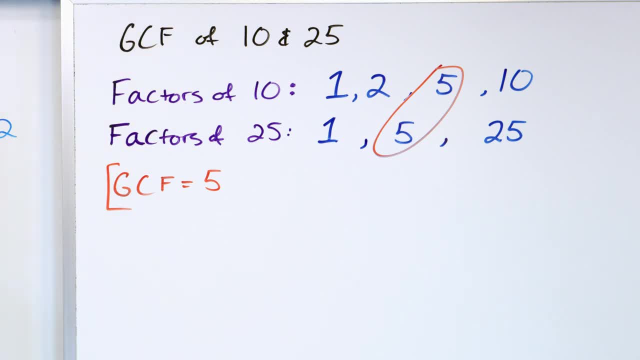 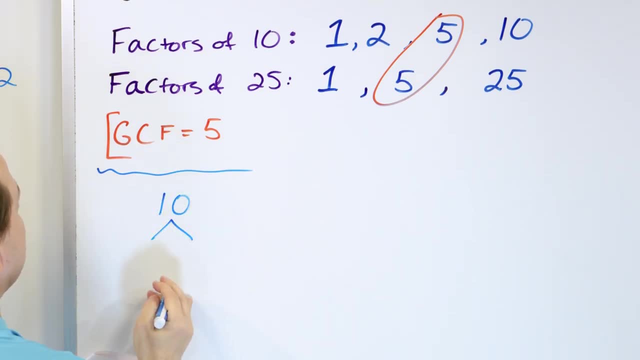 The greatest common factor of that is equal to 5.. Now we're going to practice the tree method to figure out the factors, because it'll be helpful for bigger problems. Let's take a look at the number 10.. What times? what gives me 10?? 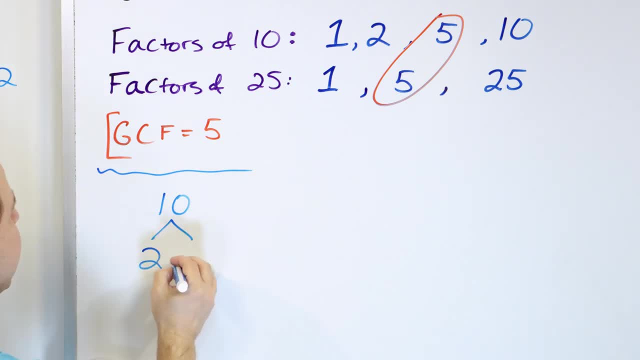 You can pick whatever you want other than 1 times 10.. So 2 times 5,, that gives me 10.. Now how can I split these further? Well, The tree is pretty much done already because, yes, 1 times 2 is 2, and 1 times 5 is 5,. but 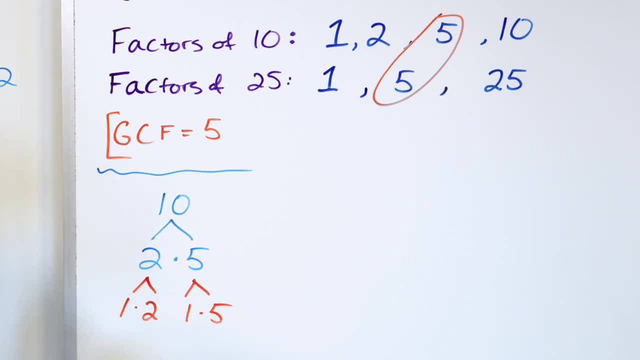 you see, I continue getting the same numbers. 2 and 5 are what we call prime numbers, because they can't be broken apart anymore other than to say 1 times 2 is 2 and 1 times 5 is 5.. So that's the tree. 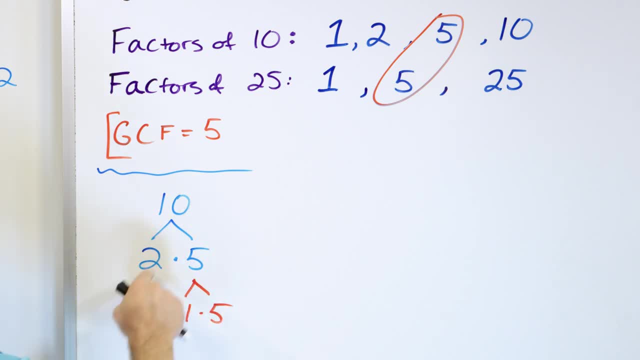 So the factors are going to come straight out of the tree. We know the number 1 is a factor. We know the number itself, 10, is a factor. The only other numbers in the tree are 2 and 5, and they're both factors. 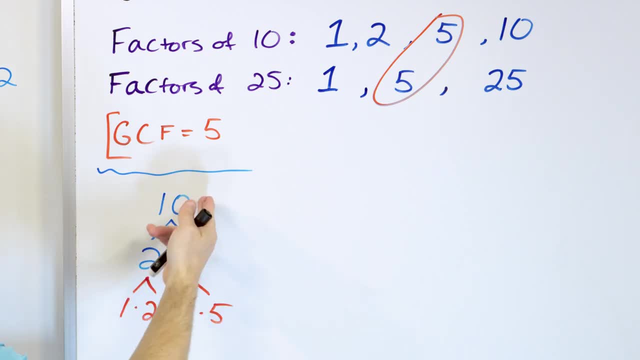 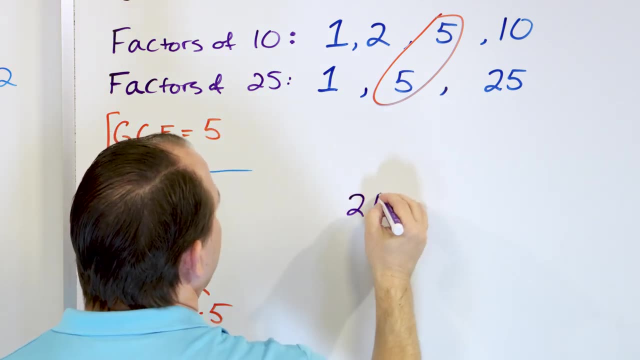 And we can multiply branches. But 2 times 5 is 10 anyway, and that's already in the list. So we can get the list, you know, as we did right here. Now let's take a look at the number 25.. 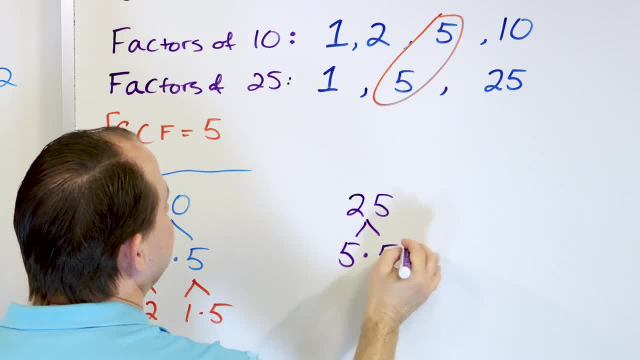 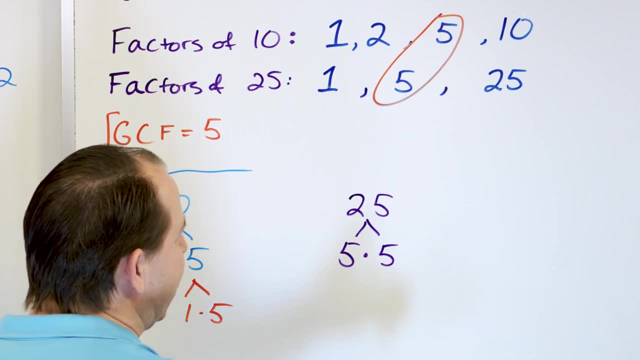 What times? what is 25?? 5 times 5 is 25.. But notice that 5 can't be broken apart anymore either. You're just going to get 1 times 5 here. So we kind of stop. We can't do any more of the tree. 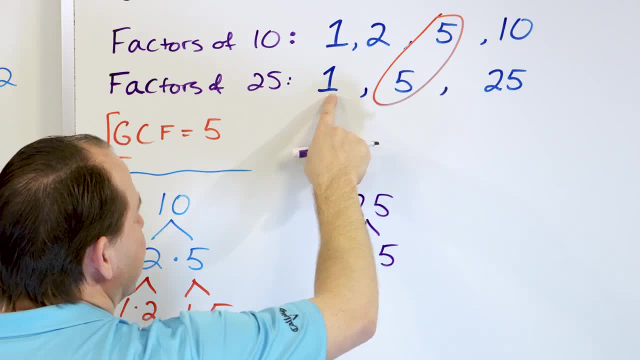 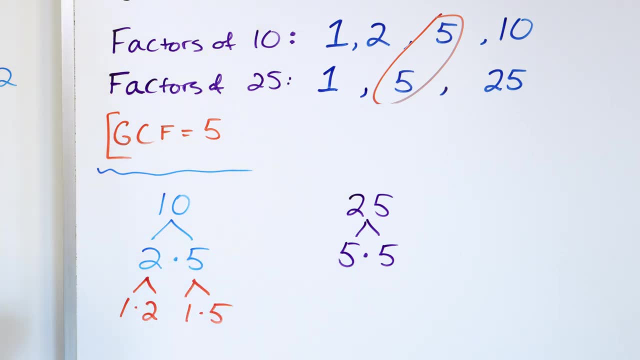 We know that 5 is going to be a factor, 1 is always a factor And the number itself is always a factor. So there's only 3 factors. There's only 3 factors for the number 25.. So these are very simple trees. 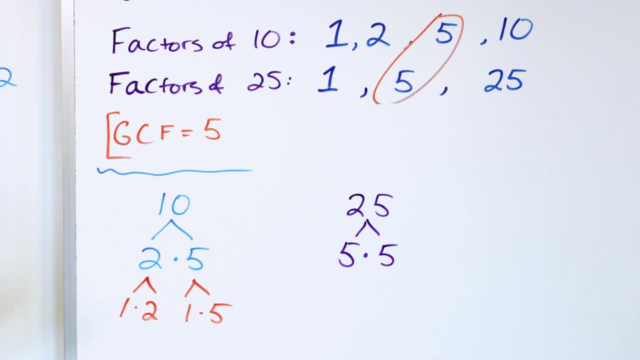 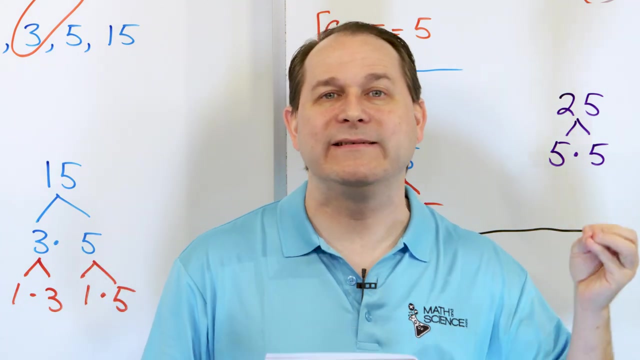 But I promise you, when we get to larger numbers, it's going to be very, very important to write the trees down, because we'll get all the factors that way. So the first two problems were what we call greatest common factor. Now we need to do a very similar problem called least common multiple. 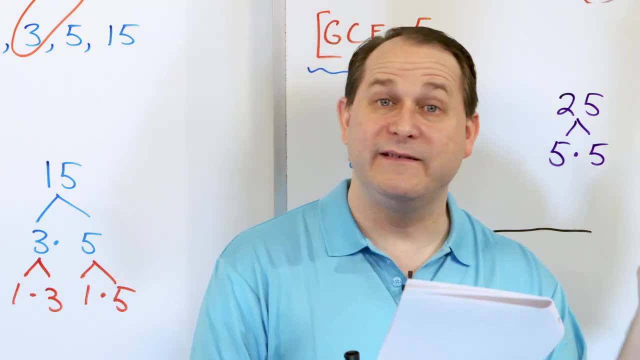 It's very often confused, but least common multiple is different than greatest common factor, And you'll see it in this video. Let's take a look, Okay. So first we need to find out why this one is the least common one. 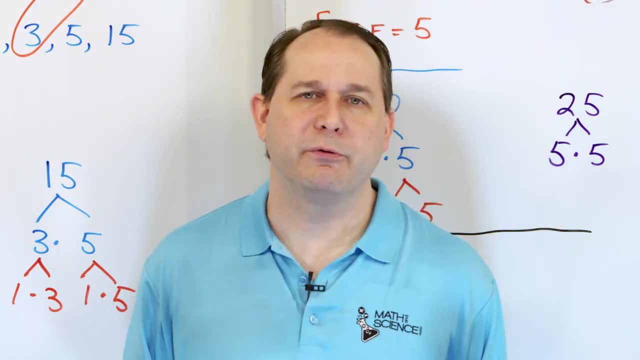 Because that's the question: What is a multiple of something? A multiple is when you skip count by the number. So what are the multiples of 2,, for instance? We can go up as far as you want. So let's say the multiples of 2 and 3 are when you count by twos. 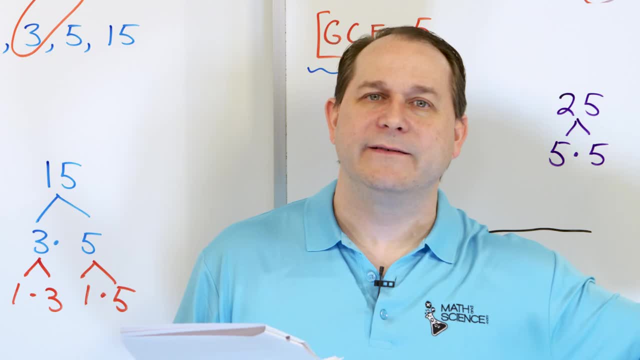 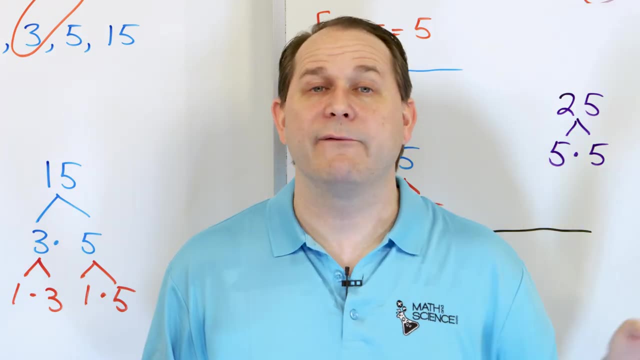 So, for instance, 2,, 4,, 6,, 8,, 10,, 12,, 14,, 16,, 18,, 20.. For every number you can go up as far as you want. The multiples of 2 go on forever. 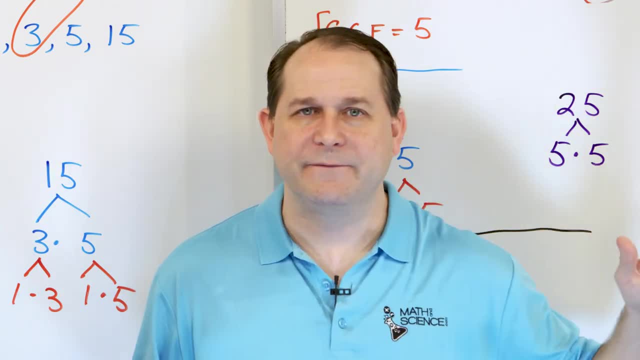 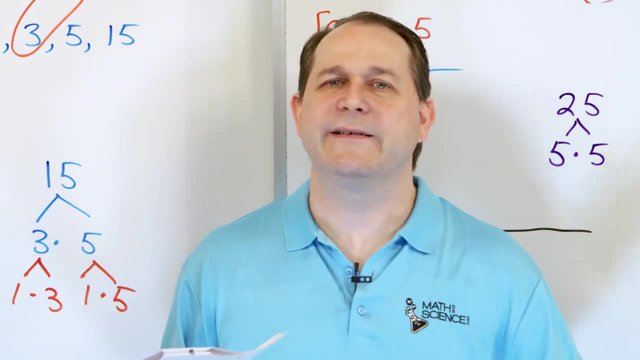 What are the multiples of 5? 5, 10,, 15,, 20,, 25,, 30,, 35,, 40.. See What are the multiples of 10? 10,, 20,, 30,, 40, 50,. all you're doing is skip counting. 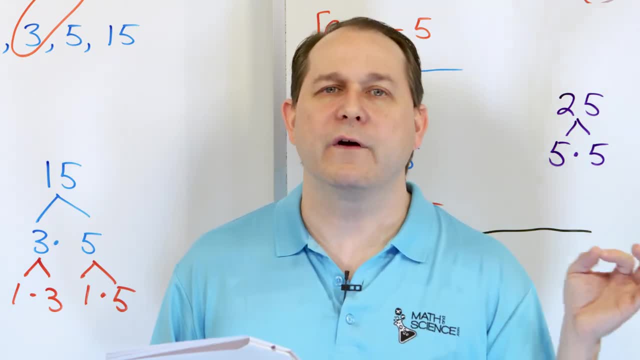 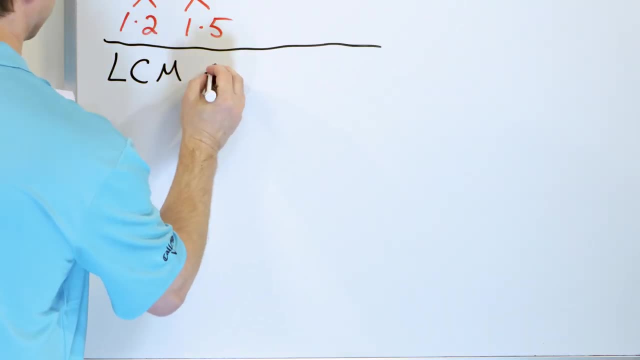 or counting by 10s or by 5s or by 2s. Those are the multiples. So in our problem here we're going to find something called the least common multiple of two and seven. So what we have to do is find the multiples of two. 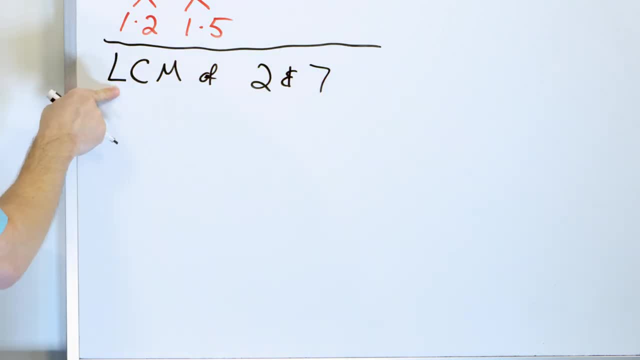 and the multiples of seven, and then we're gonna find the smallest one that's common to both. So it's very similar, but different than what we've done before. So let's find the multiples of two, the multiples of two. All right, what are the multiples of two? 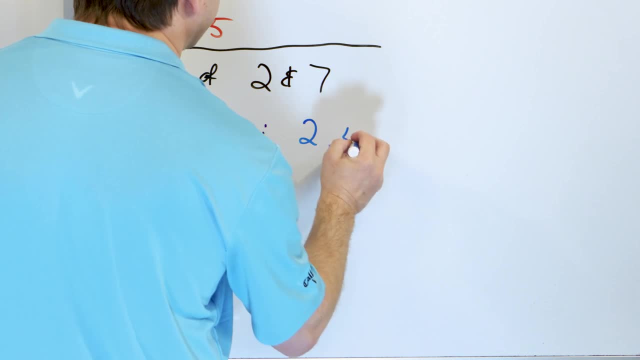 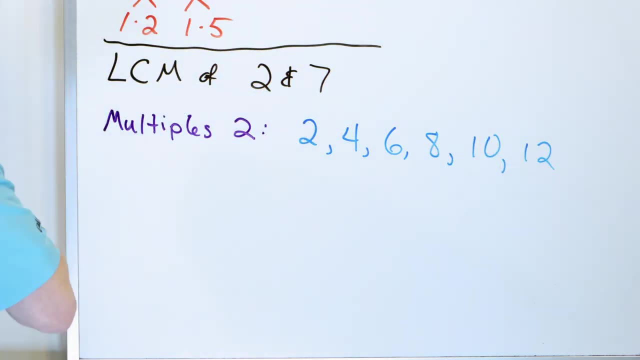 We just talked about that. Well, we can just count by twos. It's two, four, six, eight, 10,, 12.. Now you can just kind of stop, because we need to do the multiples of the other one to figure out. 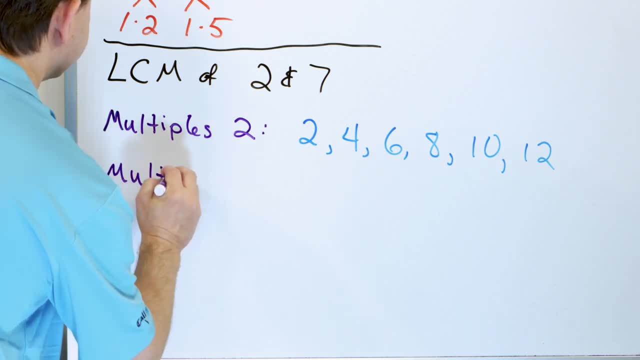 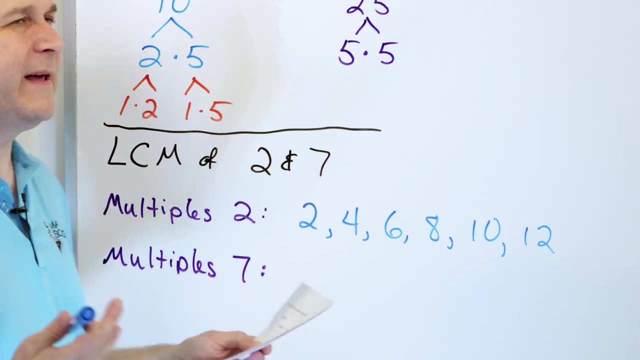 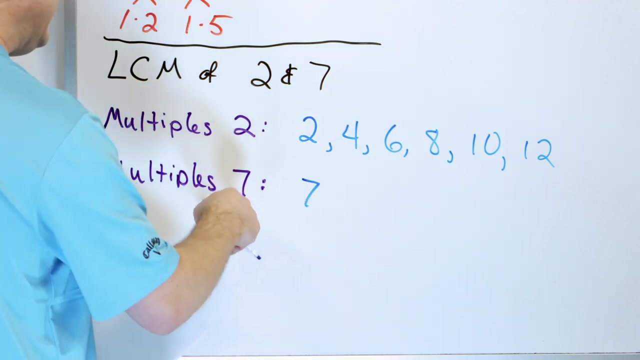 what the answer's gonna be. What are the multiples of seven? We're gonna skip count by seven. Now, you don't often skip count by sevens, but multiplication is basically skip counting. So think of it this way: Seven times one is seven, and we count by seven. 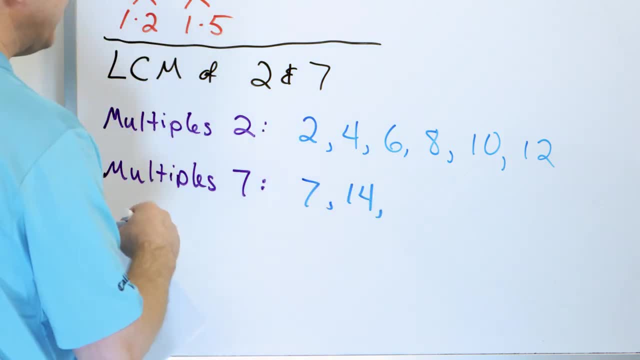 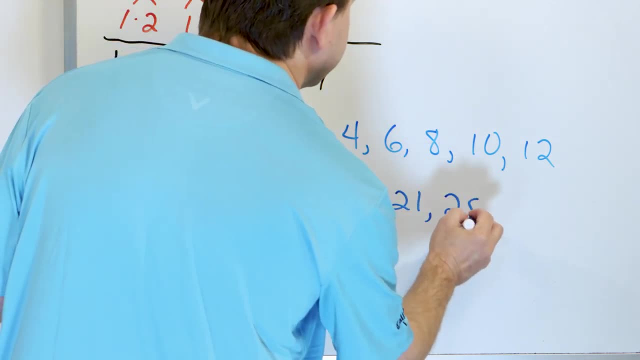 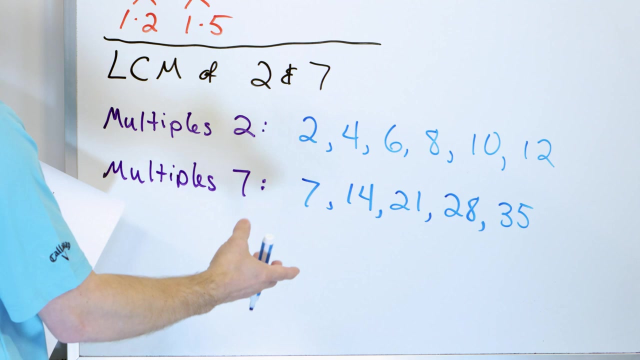 Seven times two is 14.. Seven times three is 21.. Seven times four is 28.. Seven times five is what? 35. So this is basically skip counting by sevens, which is multiplication. Seven times one is seven. 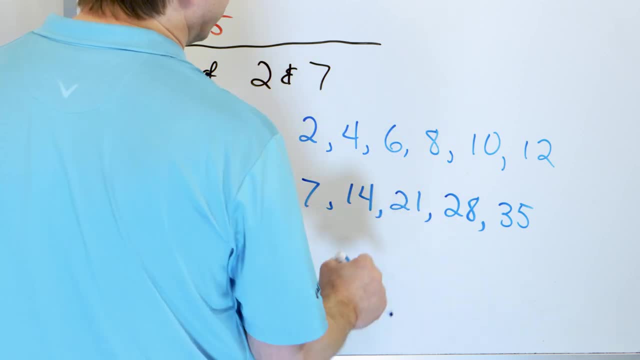 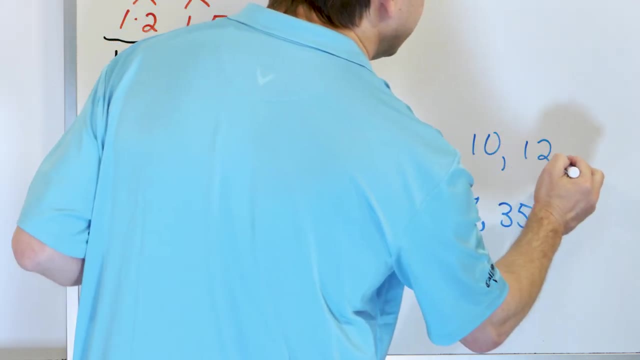 Seven times two is 14.. Seven times three is 21.. Seven times four is 28.. Seven times five is 35. We don't see anything in common yet. but then we realize, if we keep going in this list, two, four, six, eight, 10,, 12,. 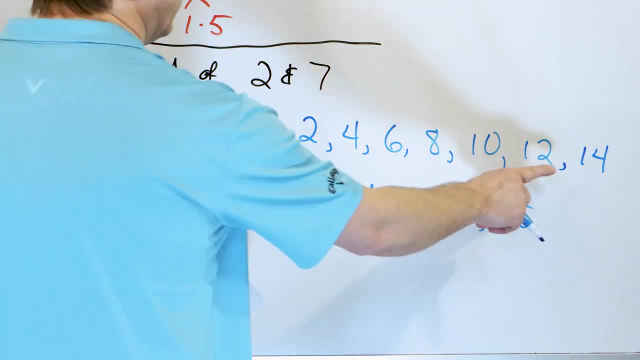 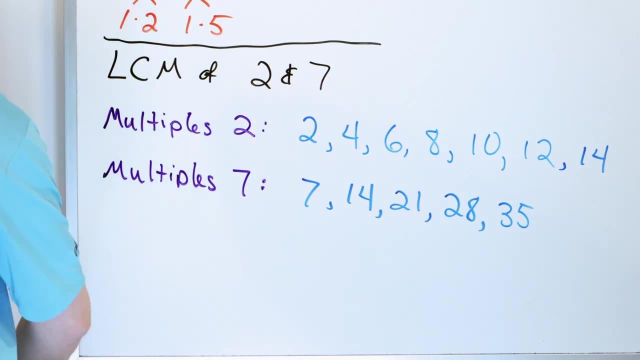 the next number is actually 14.. And 14 is common to both. And notice we're looking for not the biggest thing that's common, the least common, the smallest thing that's common. So basically, this number is the smallest number that is common to both lists. 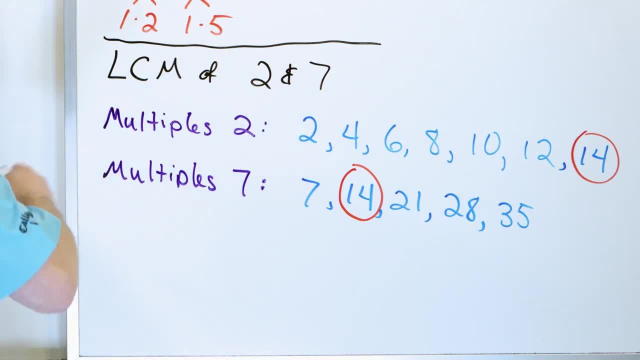 The smallest number common to both lists. So the least common multiple of these two numbers is actually 14.. The least common multiple of these two numbers is 14.. And, honestly, least common multiple is a little easier to deal with because you don't have to do. 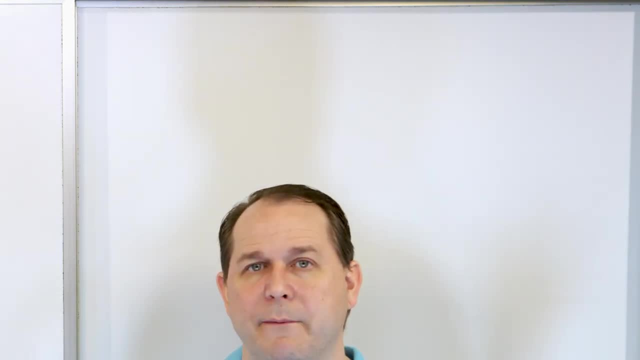 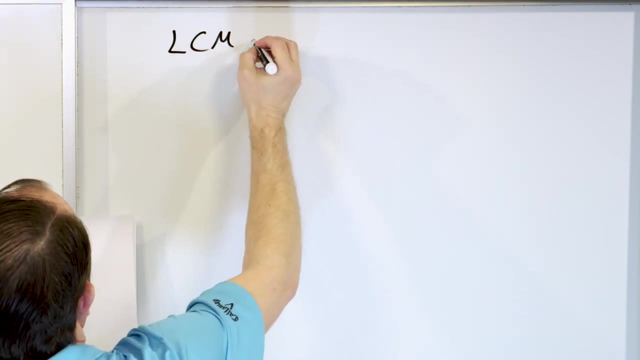 any factor- trees or anything. So we're going to be doing a bunch more of these problems to give you the hang of it, And we'll also be able to speed up a little bit as we go. Let's find the least common multiple of four and 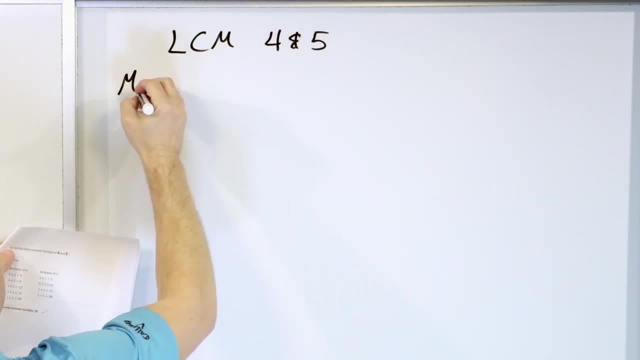 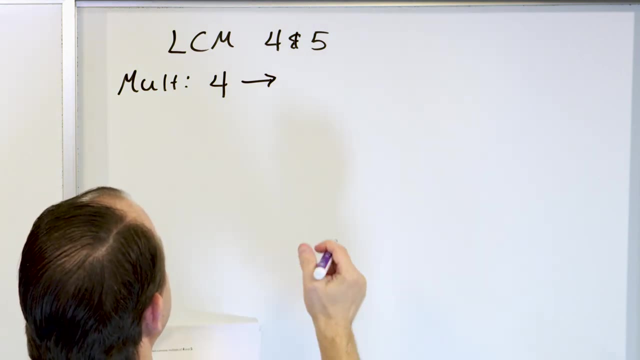 and five, the number four and five. So let's take a look at the multiples of the number four. Multiples of the number four. We just count by fours. Four times one is four. Four times two is eight. Four times three is 12.. 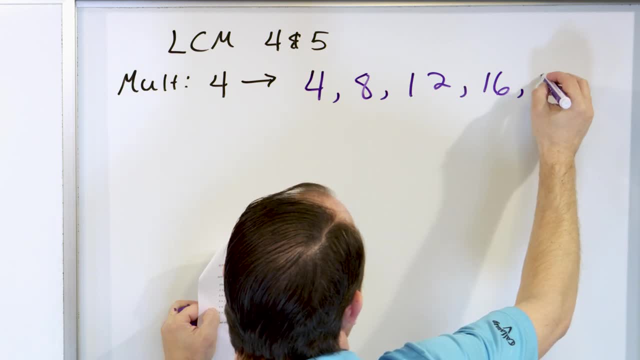 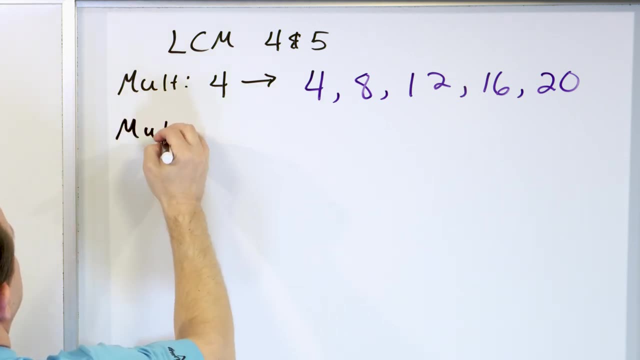 Four times four is 16.. Four times five is 20.. Now you can keep going, but let's just see what we get with the other list first. What are the multiples of five? What are the multiples of five? We count by fives. 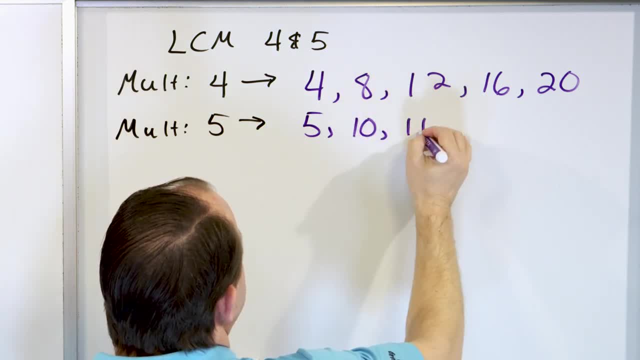 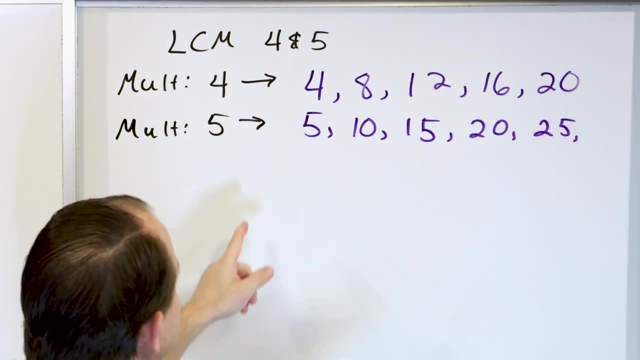 That's easy Five: 10, 15,, 20,, 25,, and it would be 30 and 35,, 40, and so on. What is common to both of these lists? When I look at them, the only thing that's common. 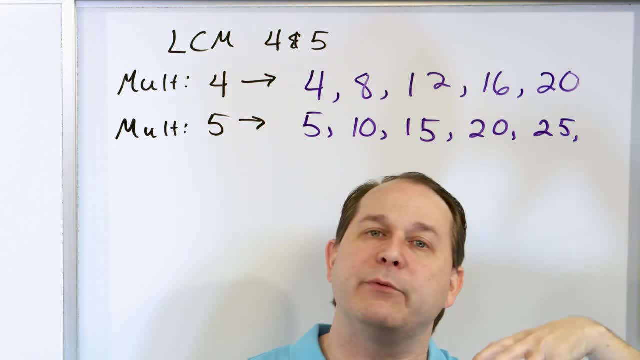 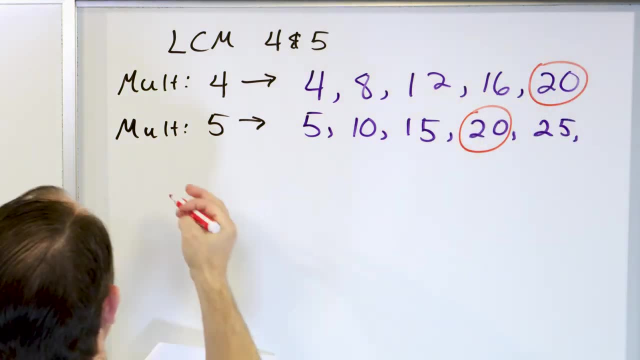 is 20 here and 20 here. I could continue the list and I would get more numbers that were common, but I can already see that the smallest one that's common to both lists is actually 20.. So the least common multiple is actually in this problem. 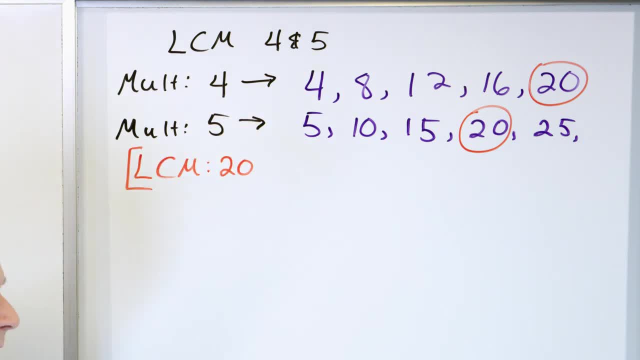 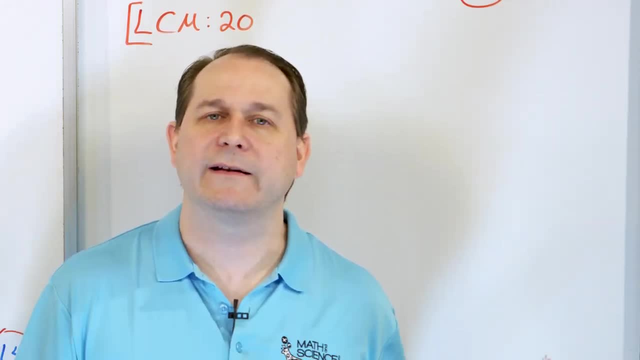 20. So greatest common factor, least common multiple. Now we're going to continue working more problems and do it using our trees and things and just kind of getting more practice, and we'll probably speed up a little bit just to kind of get more practice. 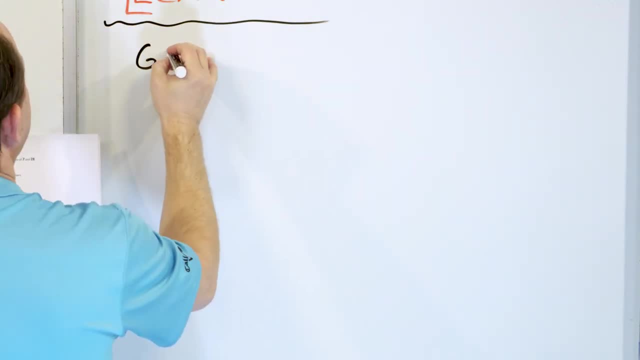 So now we're gonna bounce back to the greatest common factor of seven and 28.. So these are factors, Remember factors. we have to figure out: what multiplies together to give me seven, what multiplies together to give me 28.. 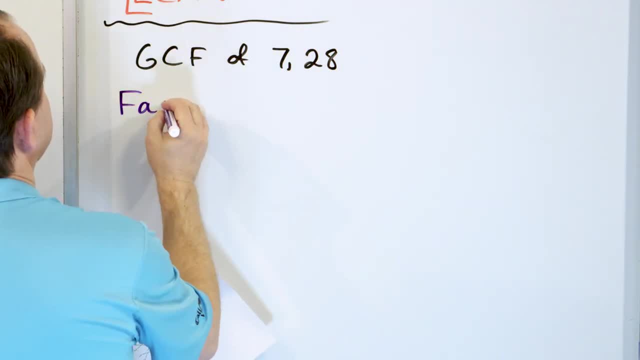 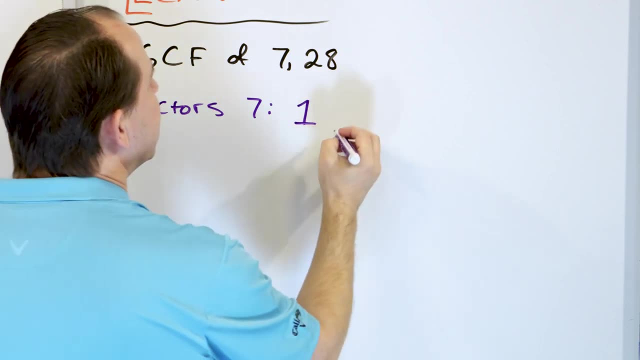 So let's figure out the factors of seven. What times? what gives me seven? Well, the number one is a factor and the number itself is always a factor. One times seven is seven, But there's actually nothing else that can multiply to give me seven. 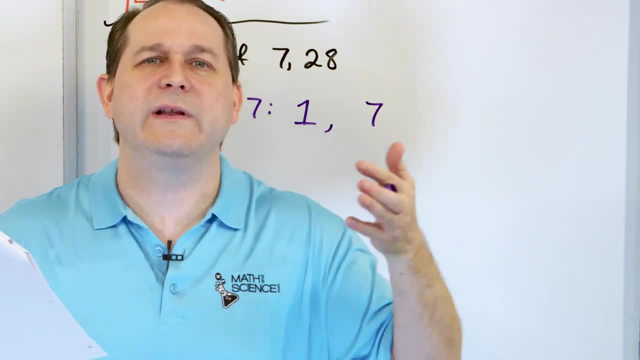 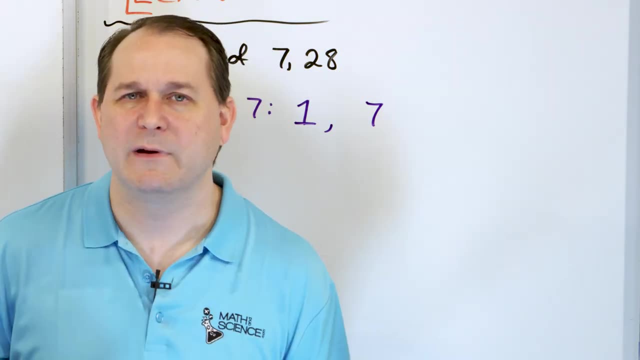 And that's what I was telling you before. When the number that you have can only be factored by saying the number itself and the number one can be multiplied to give me the number, then we call it a prime number. It can't be split apart anymore, basically. 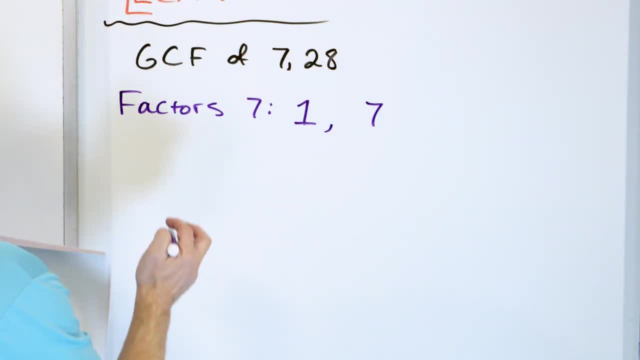 It's more basic than that. So seven is what we call a prime number. So let's figure out the factors of 28.. Now, this one's a little bit tricky because it's a bigger number. It's a bigger number, But let's use the same process: the factors of 28.. 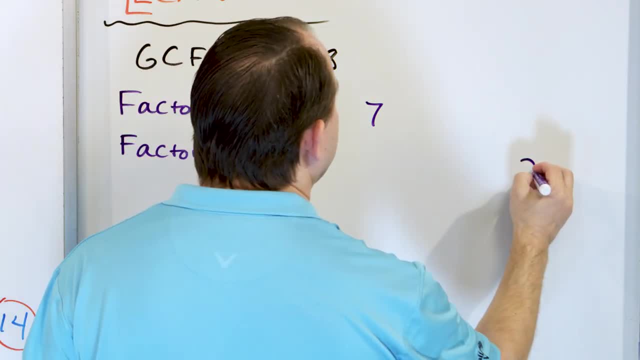 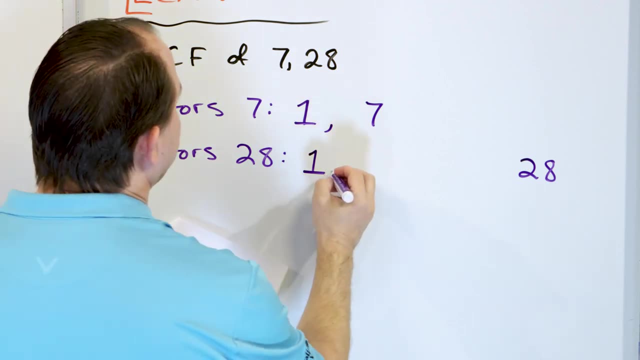 Well, the number one is going to be a factor and the number 28 is always gonna be a factor, because the number itself- one times eight, or it's one times 28- is 28.. So let's figure out what else can fit in here. 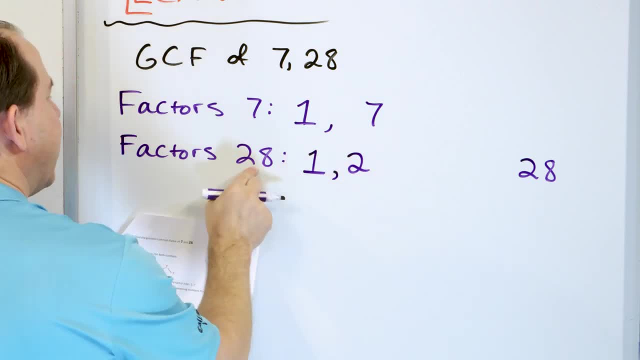 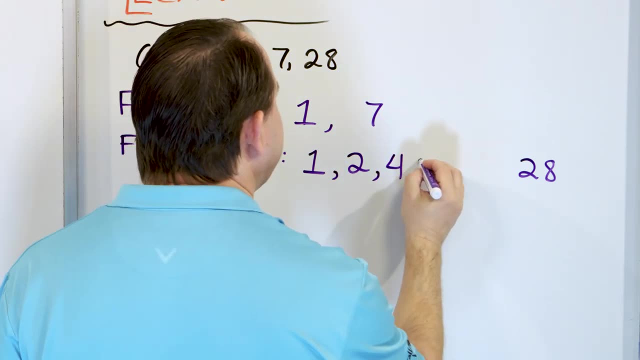 Two is a factor because this is an even number. It can divide in there, of course. Four is a factor because four times seven is 28.. And seven is also a factor because seven times four is 28.. Now, this one might be difficult for you to kind of realize. 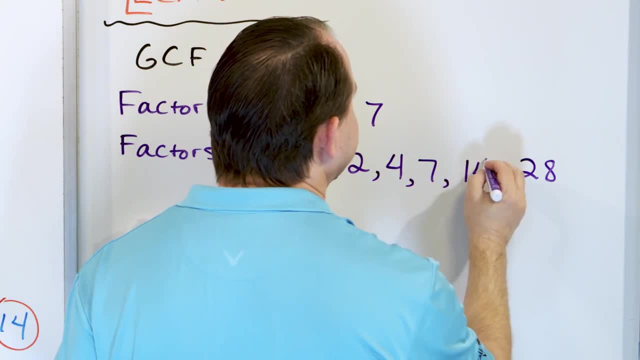 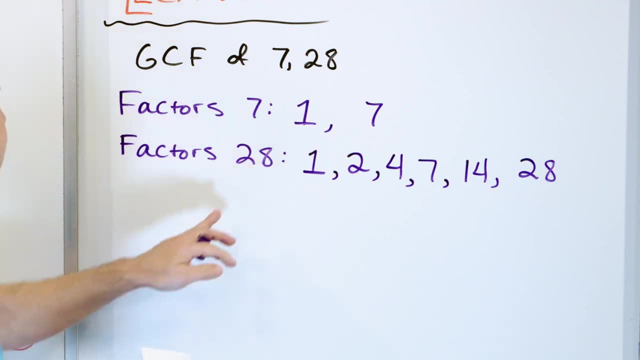 but another factor of this is 14.. 14 is a factor You know when I go up from seven, eight, nine, 10,, 11,, 12, and 13,. none of those are factors They cannot divide in here evenly. 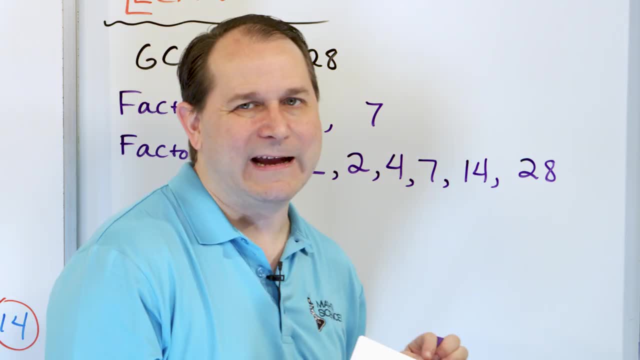 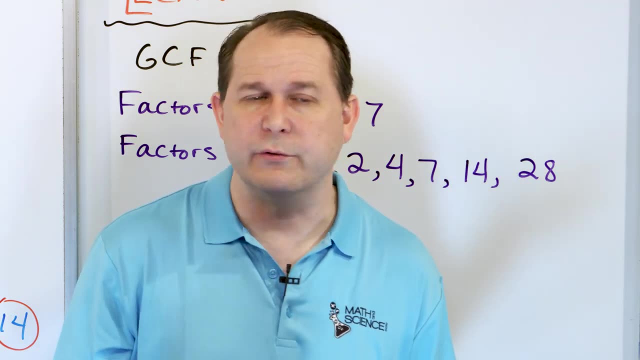 or multiply by something to give me this. But 14 can, And you may not remember that, but 14 times two is 28. And it's not something you might remember, but it's true. That's why I'm saying when the numbers get bigger. 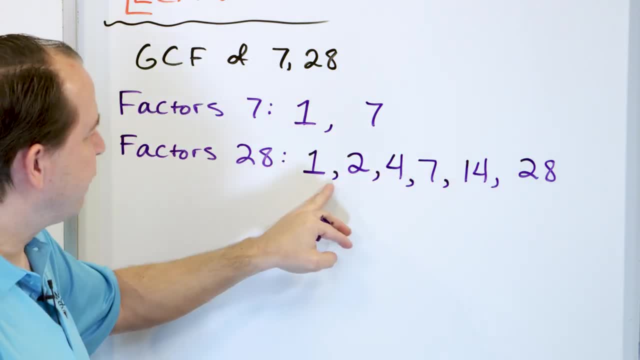 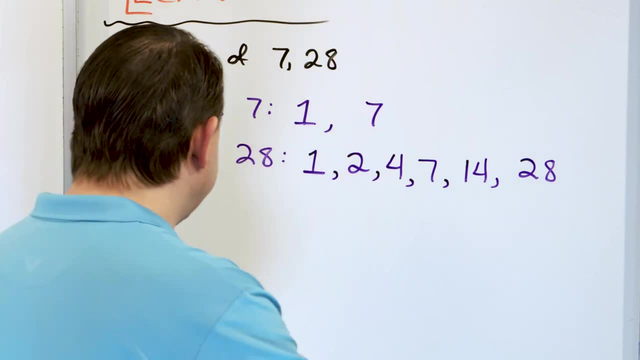 finding all of the factors might be tough, But for now, just trust me that 14 times two, when you multiply that, it gives you 28, and there's nothing else bigger than 14. that's going to work. So this is the list of factors. 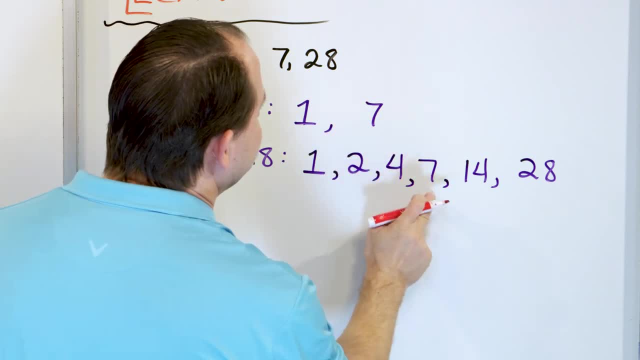 What is the commonality? One is common and seven is common, and the greatest common factor is seven. So we say the GCF is equal to. So we say the GCF is equal to. So we say the GCF is equal to. 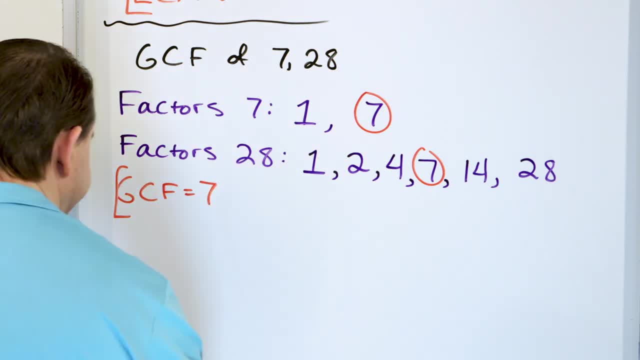 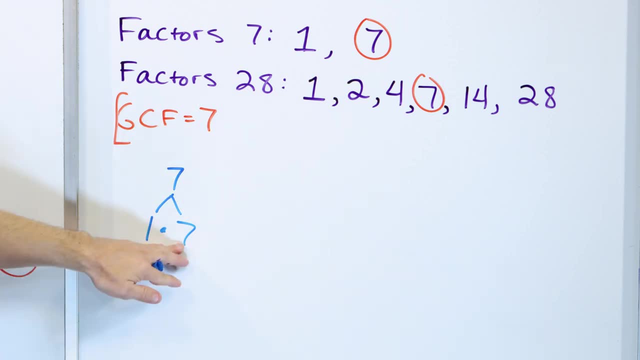 seven. Now I definitely want to do the factor tree for this. Let's do the factor trees of seven. Seven is just one times seven. There's nothing else to do. So the factors are one and seven come straight out of there. 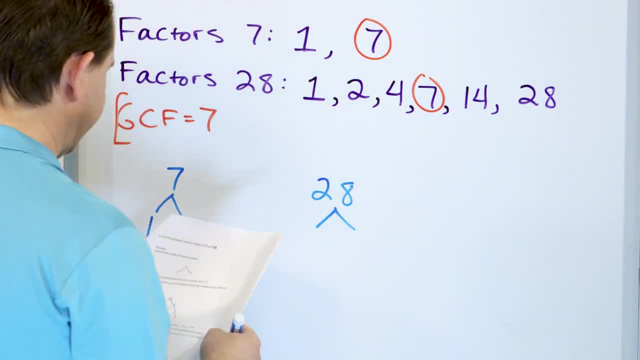 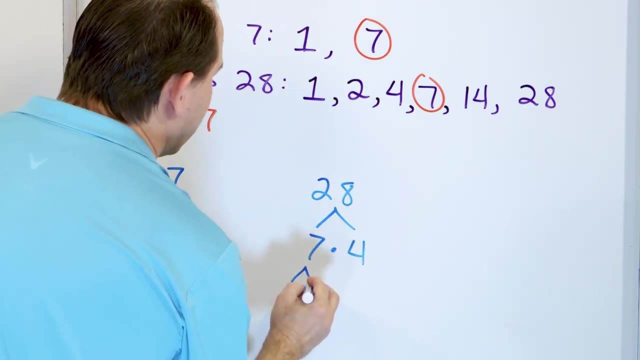 Now let's take a look at the number 28.. Let's figure out the factors here Now. I know from multiplication that seven times four is 28.. I know that seven can be broken as one times seven, but it doesn't really go any farther than that. 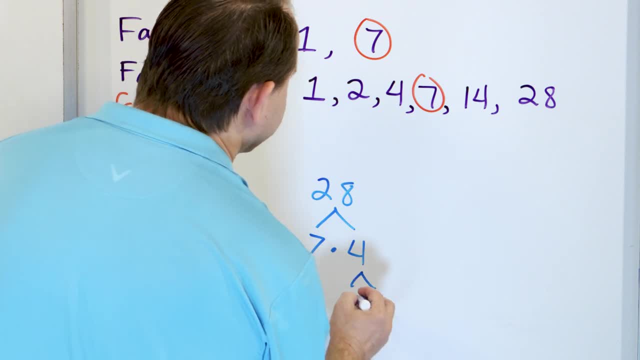 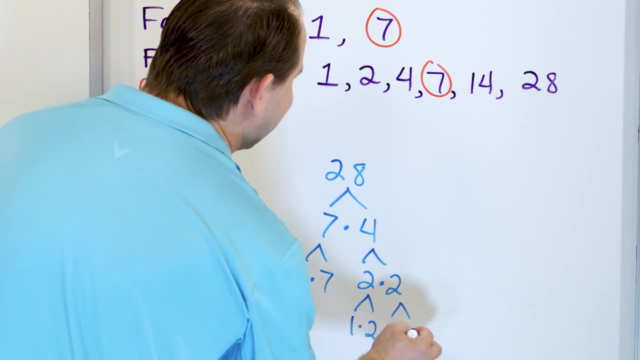 because seven is what we call a prime number And four can be multiplied or broken down into two times two, And of course the two can be written as one times two and this two can be written as one times two, but I can't go any farther than that. 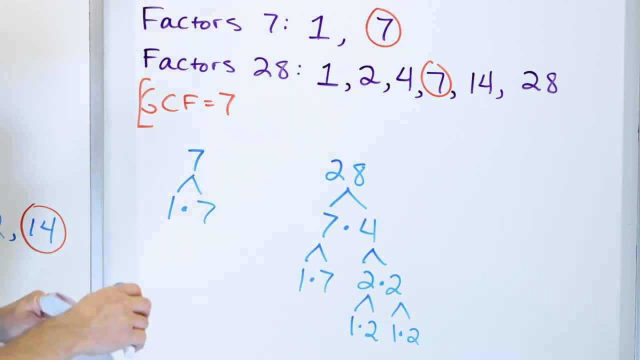 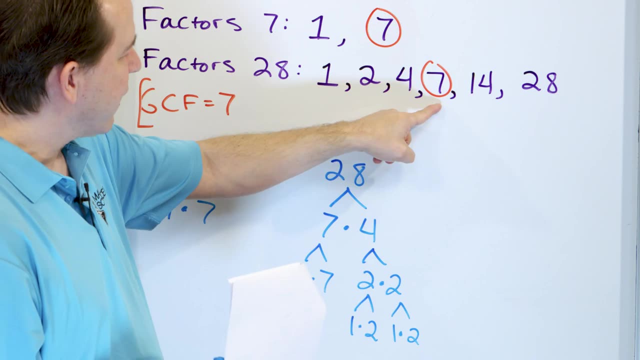 because I can't split these twos up anymore. So let's see if all the factors are here. One is a factor. Two is a factor. Four is a factor. Seven is a factor. I'm reading right out of the chart: 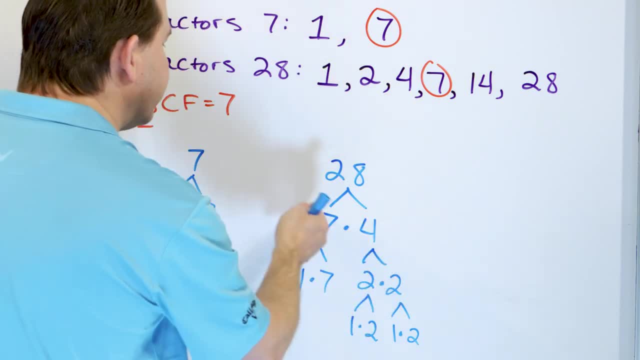 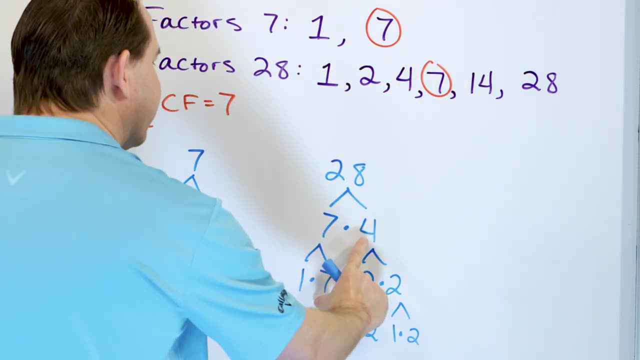 28's a factor. But remember I told you you can cross. multiply the branches Seven times two is 14.. So 14 is also a factor. If you try to multiply this way, seven times four is 28.. That's already in the list. 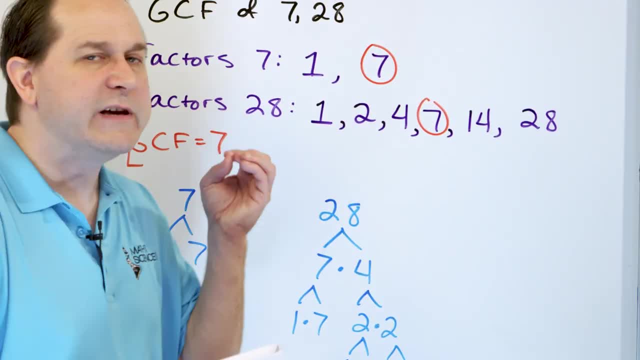 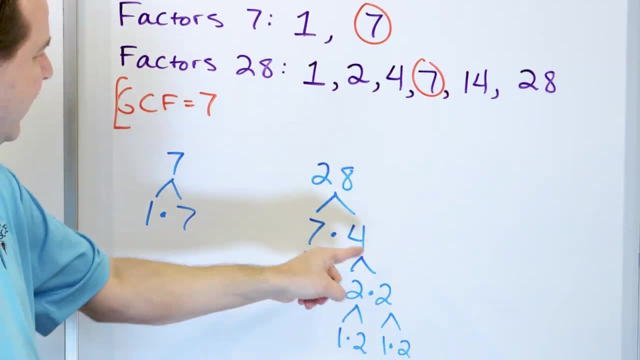 Two times seven is 14.. That's the same number as before. So you see, you can get all the factors from the tree. You read every number out of the tree and it goes into your list and you also try to cross, multiply branches. 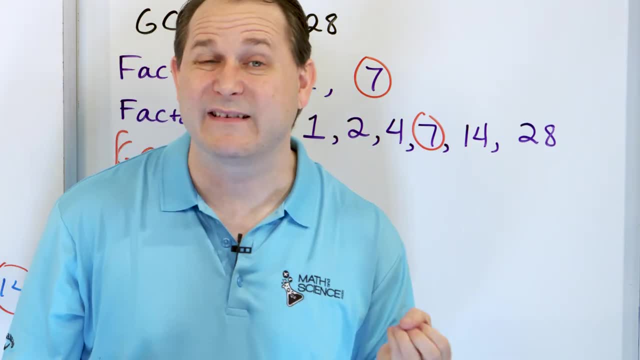 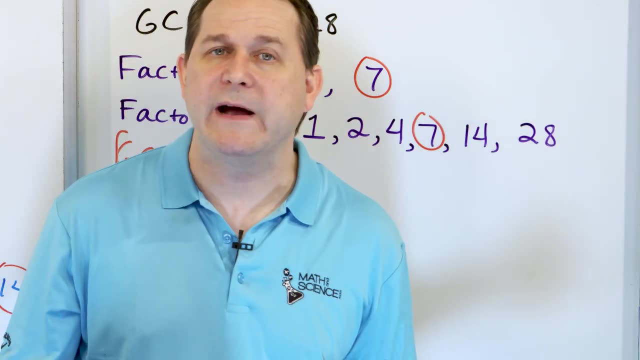 and that's how we pick up the 14.. You might have easily missed the 14 if you didn't do this, And as the numbers get bigger and bigger and bigger and the factors get more and more and more, it gets really hard to find them all, unless you use a tree. 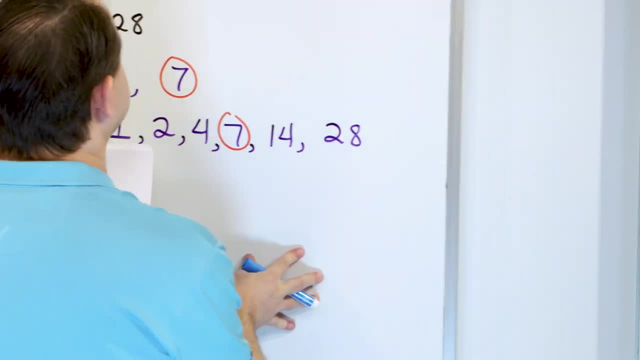 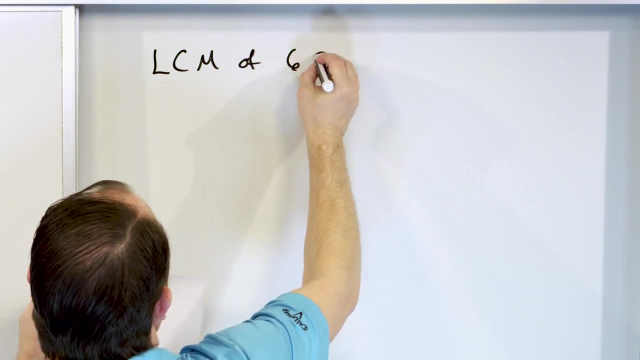 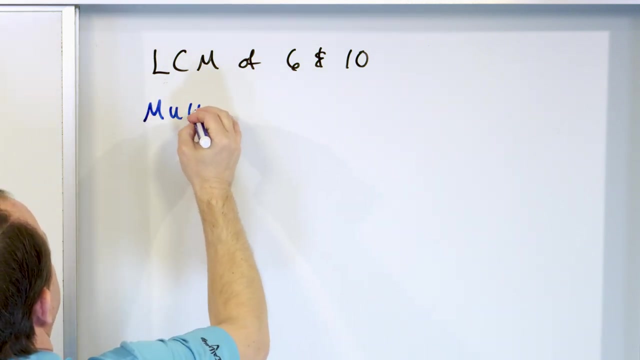 So the greatest common factor here for this problem was seven. All right. next problem: Let's find the least common multiple of six and ten. Six and ten. We need to switch back to thinking about multiples. Let's find the multiples of six. 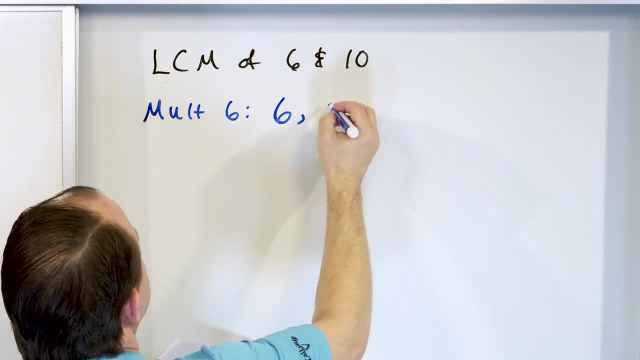 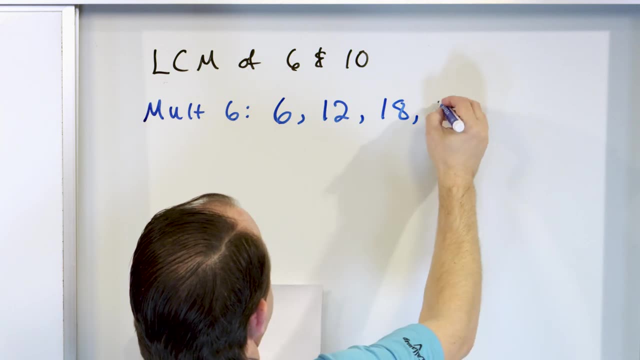 We're gonna be counting by sixes, So you can think: six times one is six, six times two is 12,, six times three is 18.. You have to know your multiplication tables. Six times four is 24.. Six times five is 30.. 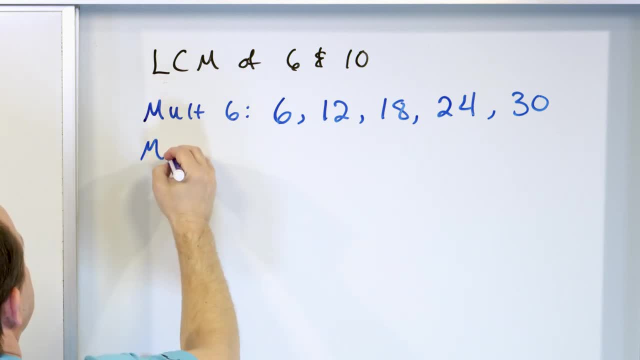 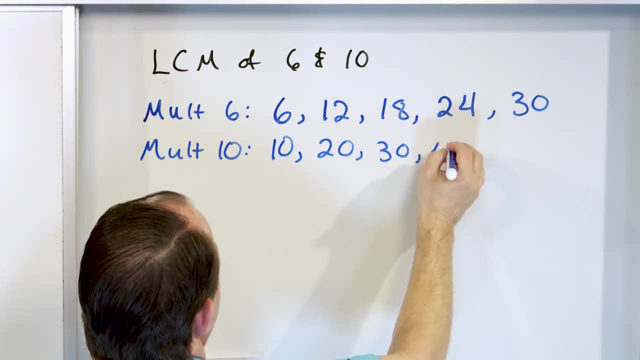 And you can keep going, but for now let's just see where the next list goes. Multiples of 10.. Count by tens. That's just 10,, 20,, 30,, 40, go, 50,, 60,, 70, and so on. 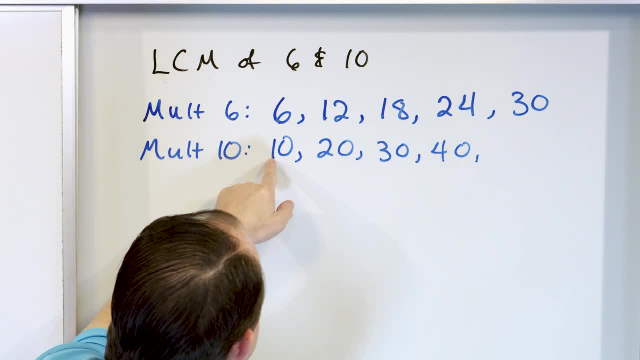 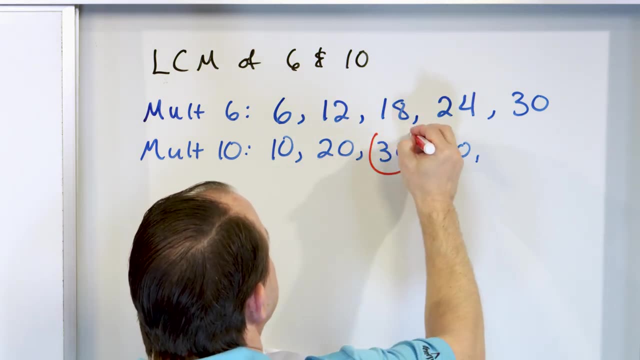 And what is the commonality here? I see 10 here, but I don't see 10 here. I see 20 here. I don't see any 20 here. 30 I see in both lists. 30 is the smallest number common to both. 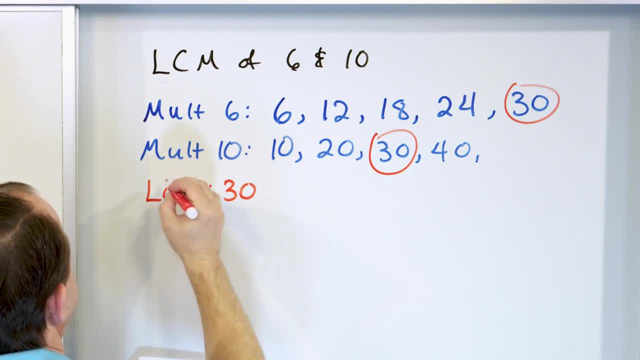 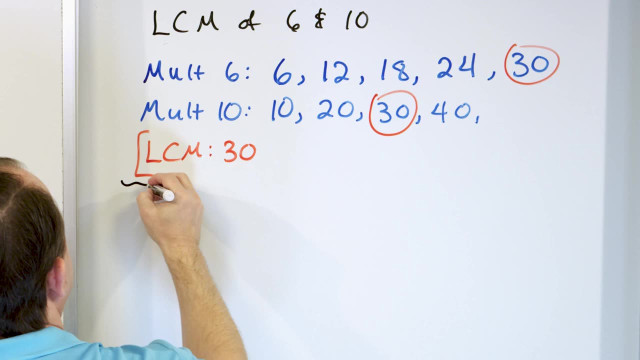 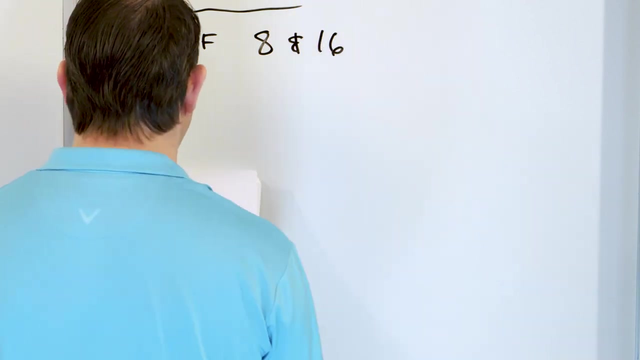 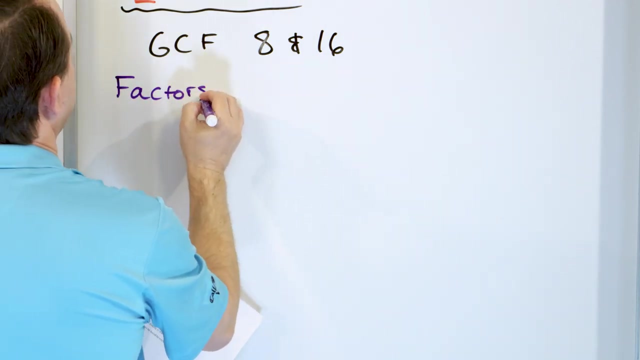 So we say the least common multiple is 30, and that's the final answer. All right, for our next problem we're gonna switch back to the greatest common factor of eight and 16,, eight and 16.. So let's find first the factors of eight. 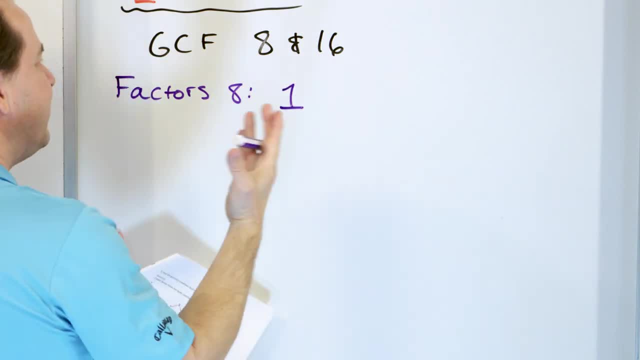 All right. what can be multiplied to give us eight? Well, the number one times eight is eight. so the number one and eight are always factors. What else? Two is a factor, because two times four is eight. Three is not a factor, but four can be a factor. 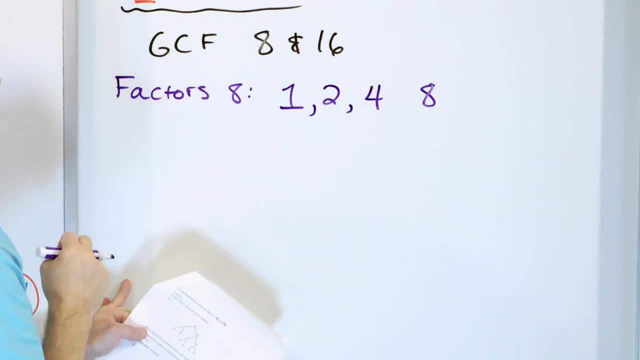 because four times two is eight. so four is a factor. What about five? That's not a factor. six, seven, those are not factors. So these are all the four factors of the number eight. What about the factors of the number 16?? 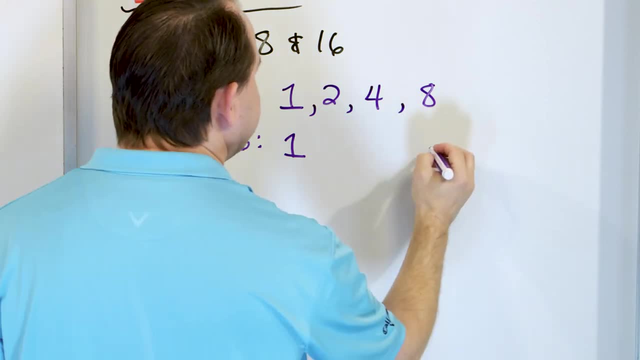 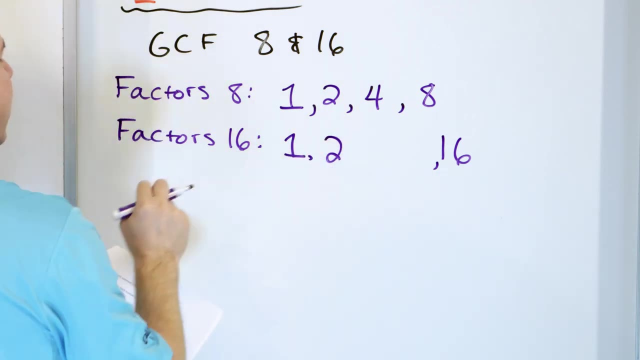 Of the number 16, well, one and 16 are always factors. The one is the number itself, because one times 16 is 16.. Two is a factor, Absolutely Yeah, is a factor, because 2 times 8 is 16.. 3 is not a factor, but 4 is a factor, because why? 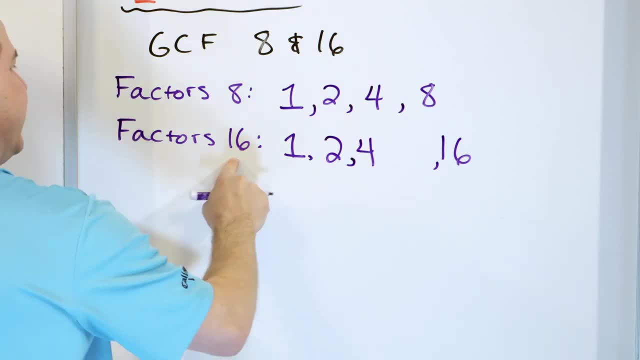 4 times 4 is 16.. 5 is not a factor, 6 is not a factor, 7 is not a factor, But 8 is a factor. Why? Because 8 times 2 is 16.. And if you go up from there, 9,, 10,, 11,, 12,, 13,, 14,, 15,. 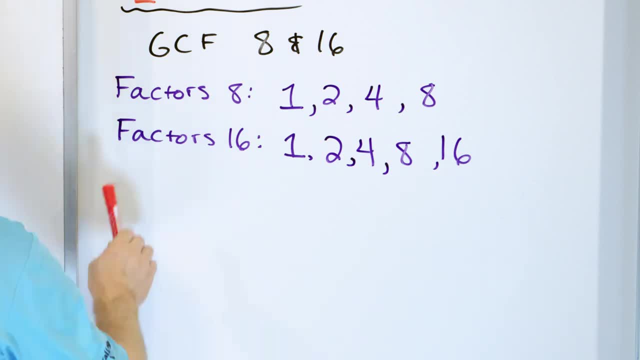 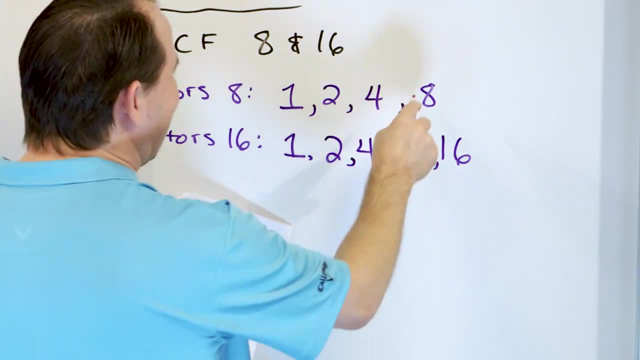 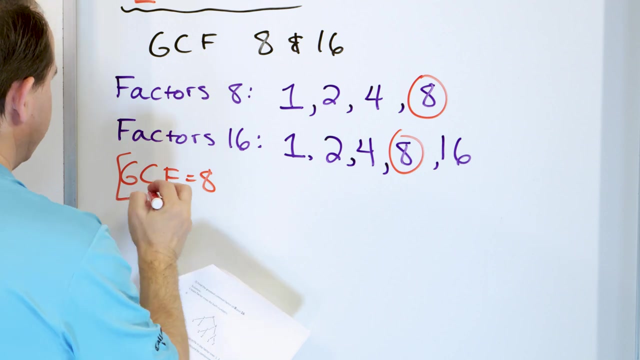 none of those are factors. They cannot multiply to give me 16.. What is the greatest thing common? 1 is common, 2 is common, 4 is common And 8 is also common, and this is the largest of the common ones. So the greatest common factor is equal to 8.. 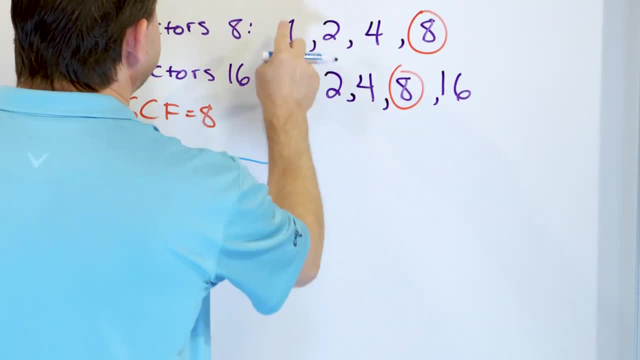 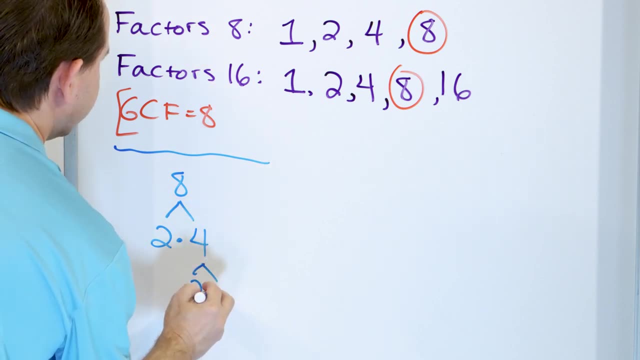 Alright, now just to get practice, we're going to use these factor trees. What about a tree for 8?? We know that 2 times 4 is 8.. 4 can be broken down further into 2 times 2.. I could. 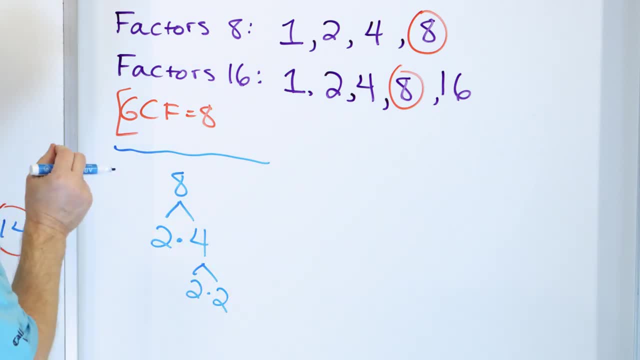 break down the 2's, but it's not going to add anything. So I look at the tree And I say 2 is a factor, 4 is a factor 1 and the number 8 are always a factor And 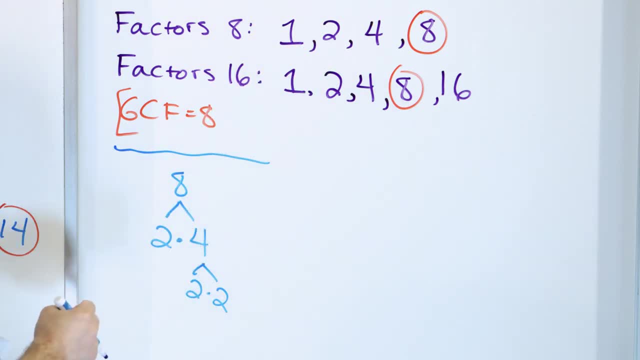 I can cross-multiply the branches 2 times 4 is 8.. That's already in there, So there's nothing else that the tree gives me. Let's take a look at 16.. Now you can do whatever you want for 16. You can do 4 times 4,, but let's just do 2 times 8.. I mean, you can pick. 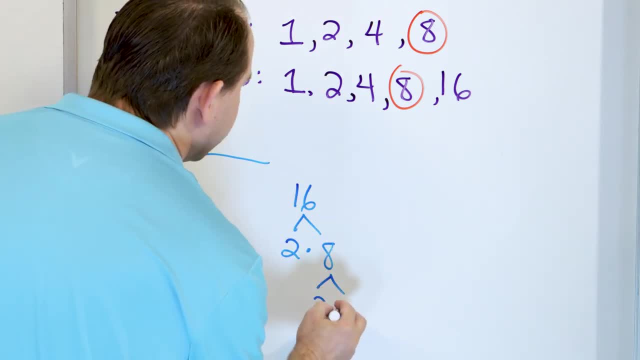 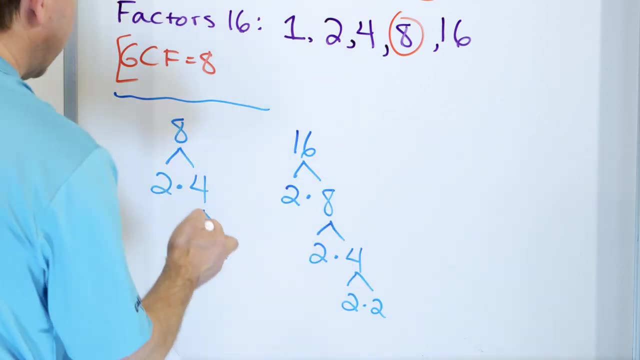 whatever you like. 8 can be further broken down into 2 times 4.. And 4 can be broken down into 2 times 2.. Now you can choose 4 times 4 and so on, but you're going to get the same place. So for: 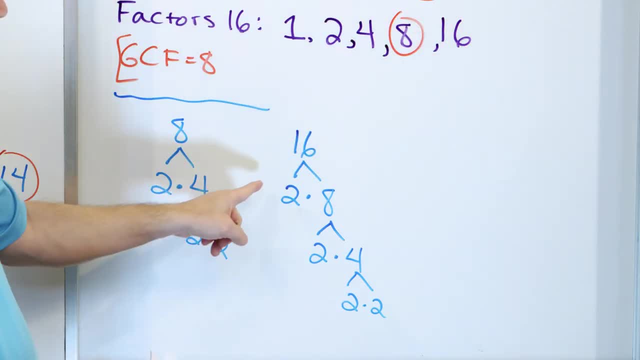 16, the number 1 and the number 16 are always factors. 2 is a factor. 4 is in the tree, That's a factor. 8 is in the tree, That's also a factor, And you try to cross-multiply 2 times. 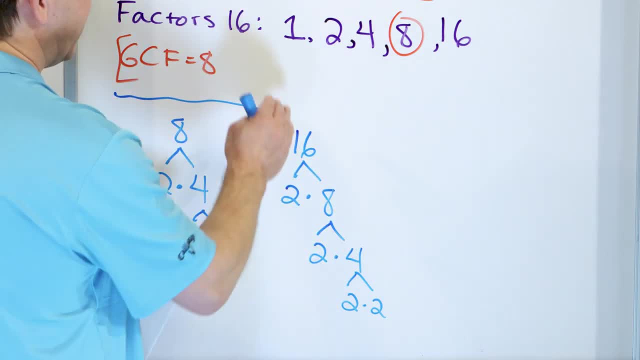 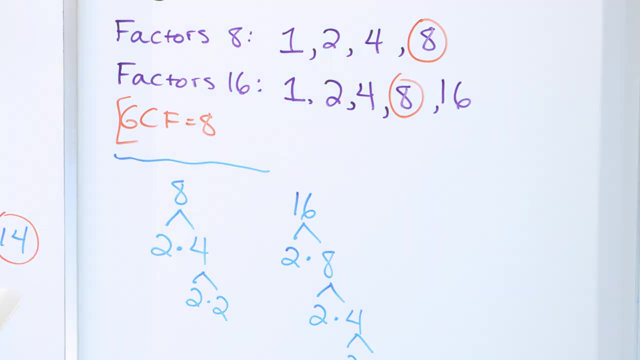 4 is 8. That's already in there And there's nothing else to cross-multiply. So these are all of the factors of 16. And so the common, the greatest common, is the number 8.. Alright, to the next problem. let's take a look at the least common multiple of. uh, sorry, not. 8.. I don't know why I had 8 in my mind, The least common multiple of 4 and 10.. So let's find the multiples of 4 first. All we need to do is skip count by 4.. So 4 times 1 is 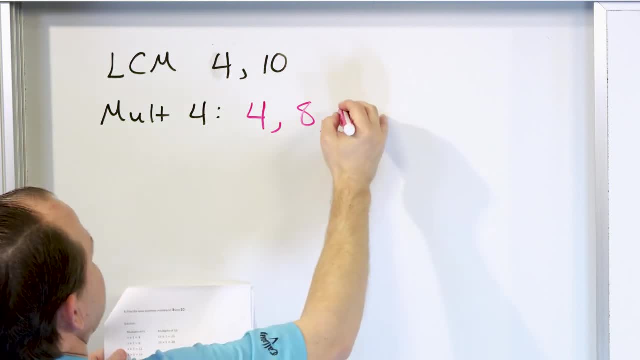 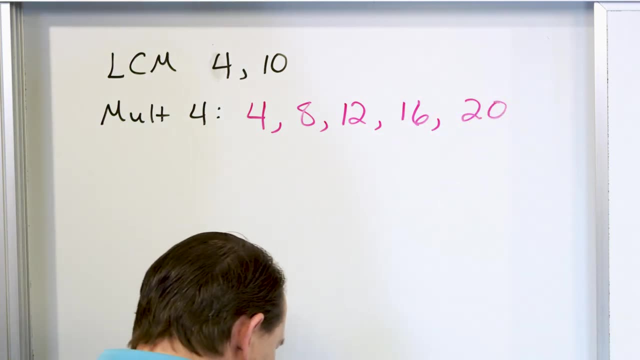 4.. 4 times 2 is 8.. 4 times 3 is 12.. 4 times 4 is 16.. 4 times 5 is 20, counting by 4's. Next we have to say what are the multiples of 10.. Now these are actually easier. Everybody. 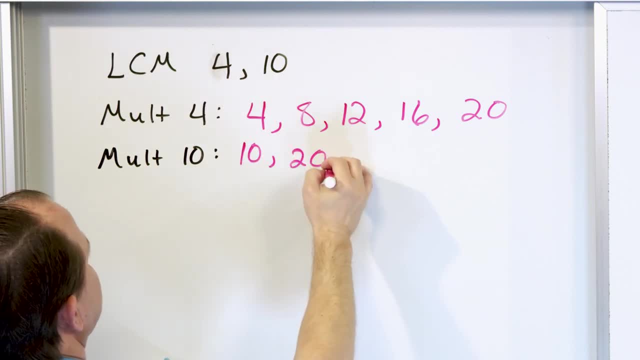 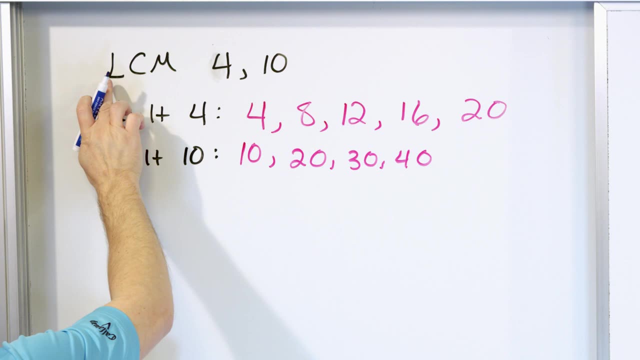 knows how to count by 10's, 10,, 20,, 30,, 40, and so on, And you can see right away that we're trying to find common things And we're trying to find the least common. Now we're. 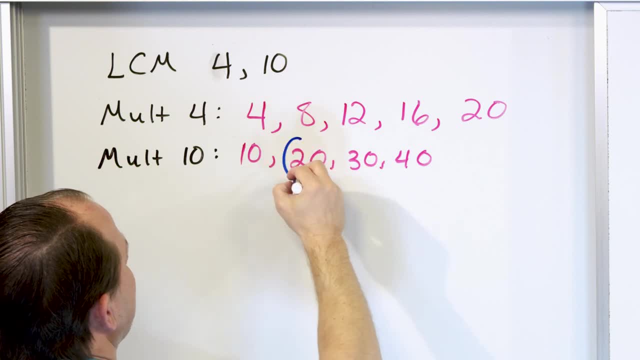 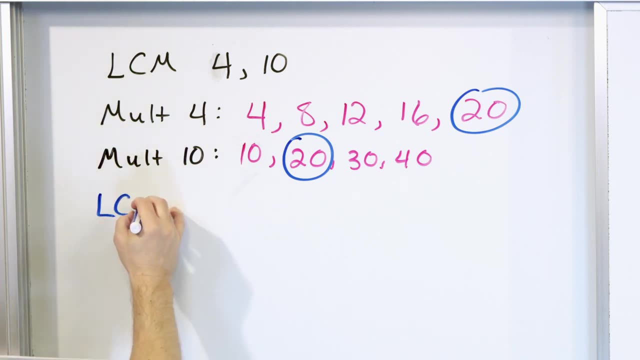 trying to find the things common and the only thing I really see is a 20, and of course that's the smallest thing that's common. None of these other numbers are common to both lists, So 20 is the least common multiple. The least common multiple is 20.. Alright, next problem. Only two more problems actually. 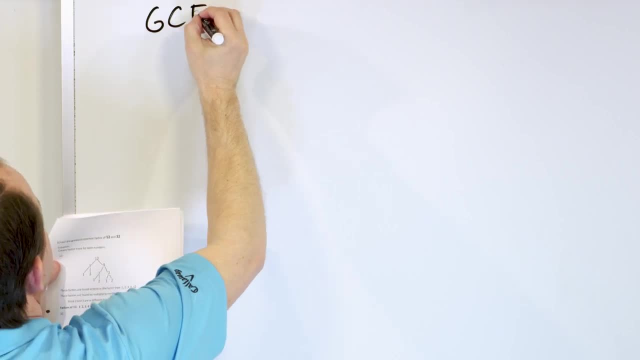 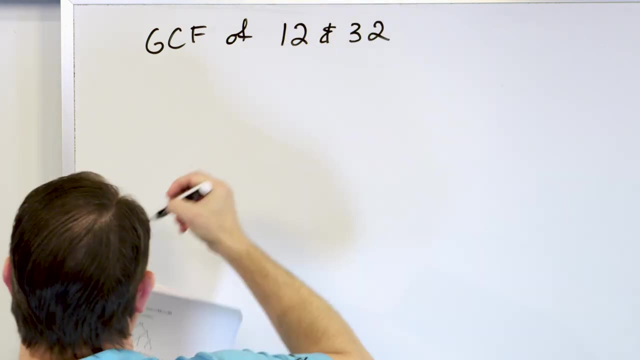 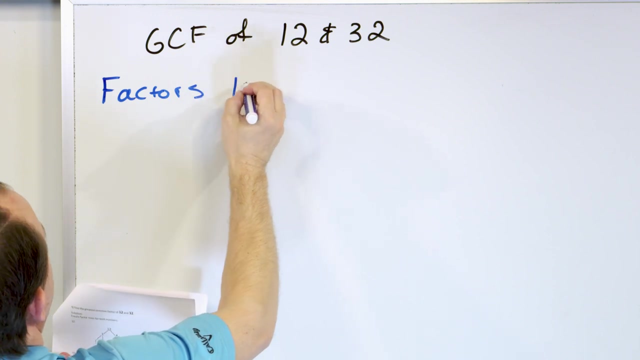 Let's take a look at it over here. Let's find the greatest common factor of 12 and 32.. 12 and 32.. So what I think I want to do here is: let's find the factors of 12 and let's. 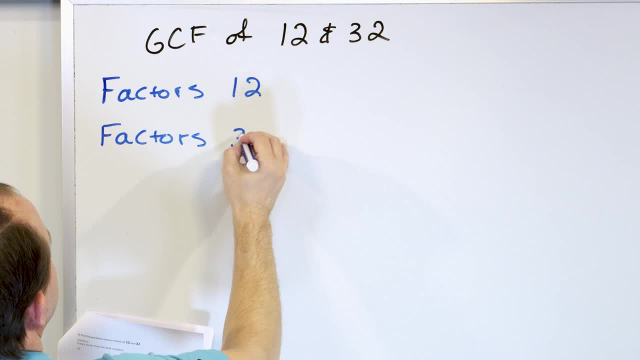 find the factors of 32.. So let's find the factors of 32.. But you see how 32 is kind of a large number. I think I want to use the factor tree straight away for this problem. Let's do it for 12.. So 12.. 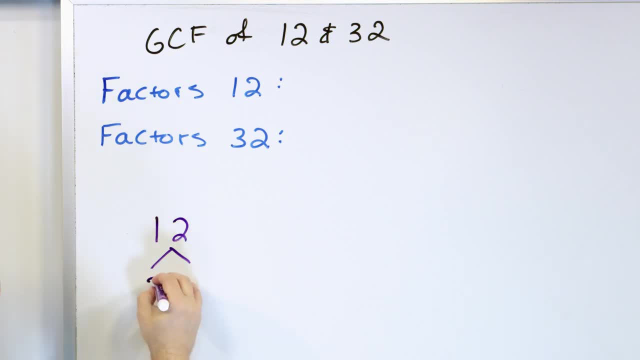 What times? what is 12?? You can do 2 times 6.. But let's just do 3 times 4.. 4 can be broken down into 2 times 2.. But you see, I can't break 3 anymore. It'll be just 1 times 3.. 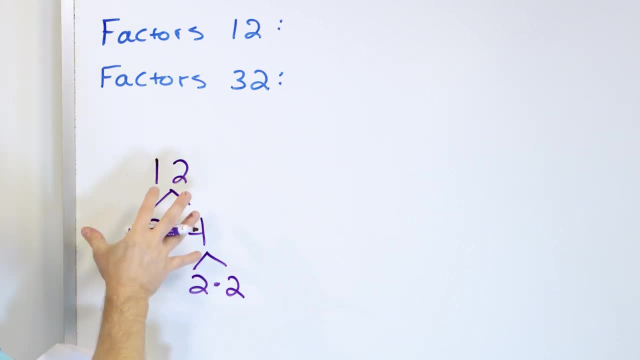 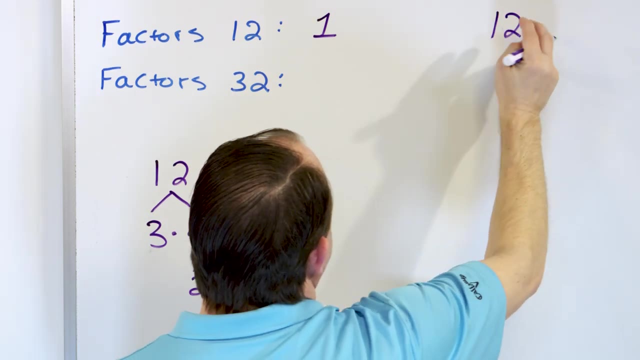 And 2. I can't break anymore because it's just going to be 1 times 2.. So I can write them if I want, but I don't need to. I know that the number 1 is a factor, That the number 12 is. the number itself is always a factor. 1 times 12 is 12.. Now 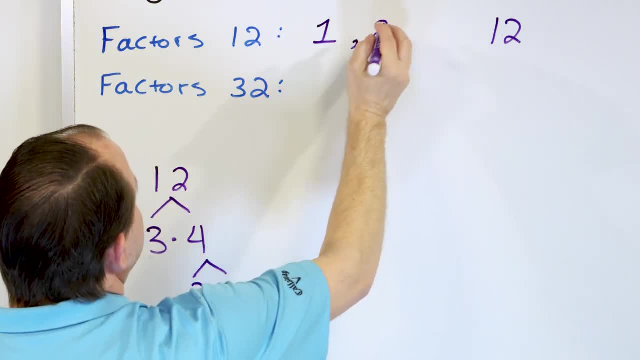 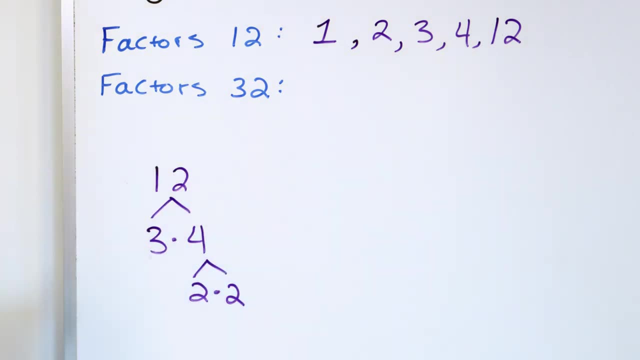 what else comes out of this tree? The number 2 is a factor. comes straight out of the tree. The number 3 is a factor. comes right out of the tree. The number 4 is a factor. comes right out of that tree. Now I cross, multiply branches. 3 times 2 is 6.. That's another factor. 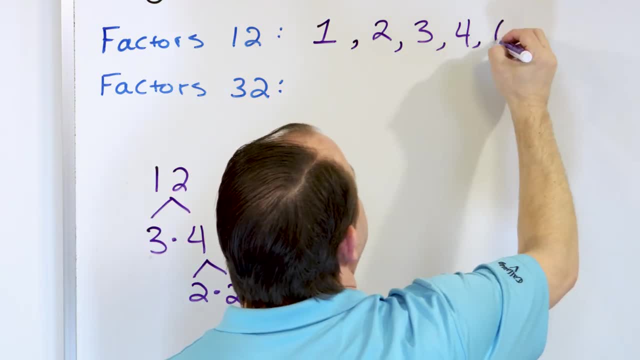 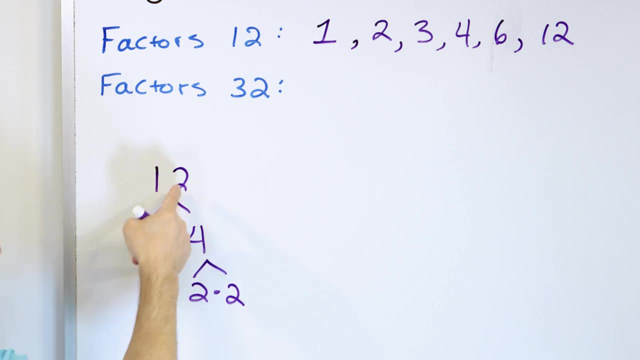 So what I'm going to do is scoot this 12 over here. 6 is also a factor, Alright. And also you can try: 3 times 2 is 6.. 4 times 3 is 12.. That's already there. 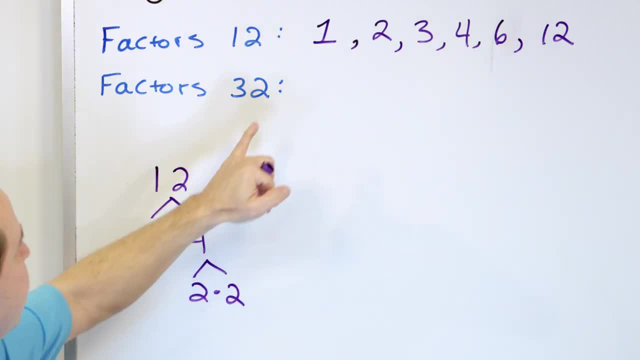 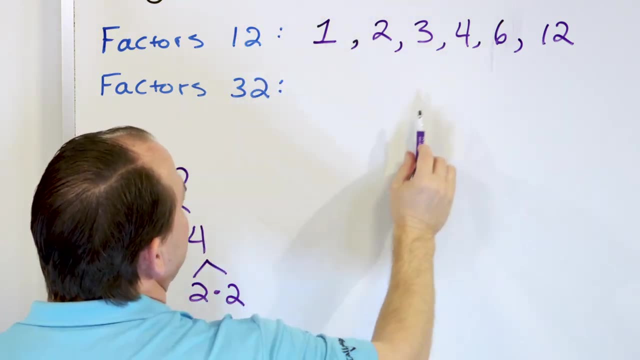 So we read all the numbers out, put them in and cross, multiply branches. These are all of the factors. Make sure you agree. 2 times 6 is 12.. 3 times 4 is 12.. 4 times 3 is 12.. 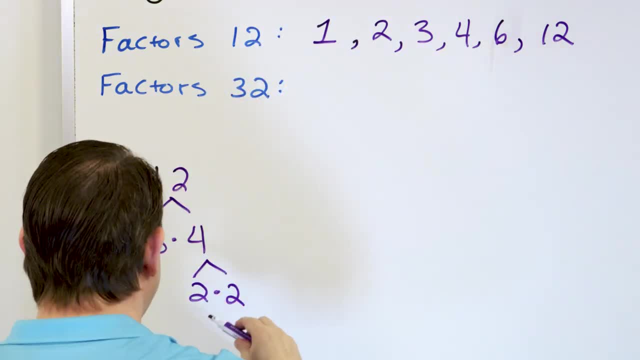 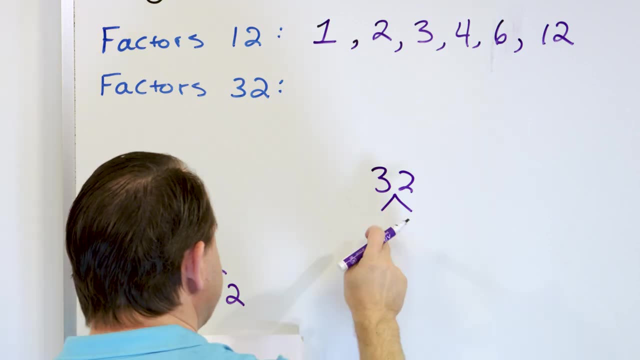 6 times 2 is 12.. And 12 times 1 is 12.. So these are all of the factors. Now let's take a look at the factors of the number 32.. So this is a larger number. You can pick whatever you'd like, but let's just do: 4 times 8 is: 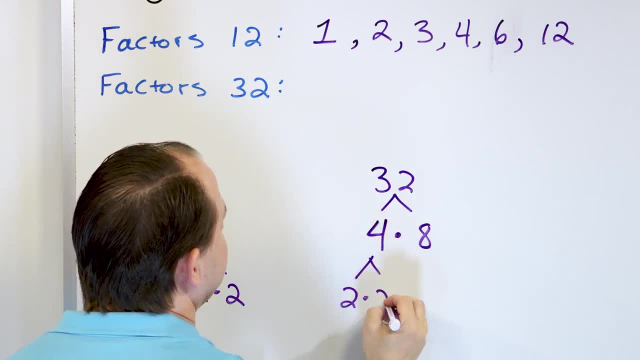 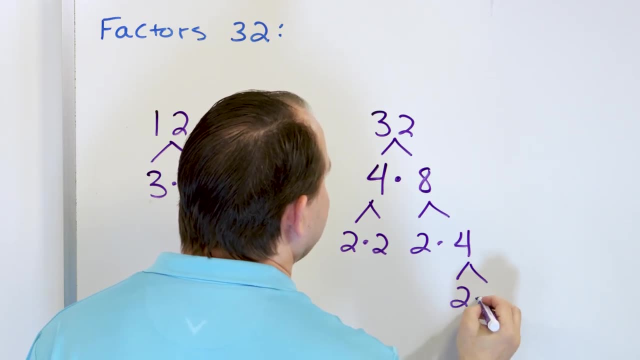 32.. Now the 4 can be broken down into 2 times 2.. The 8, you can break it down into 2 times 4.. And the 4, you can break this down into 2 times 2.. You see how I get it all down to. 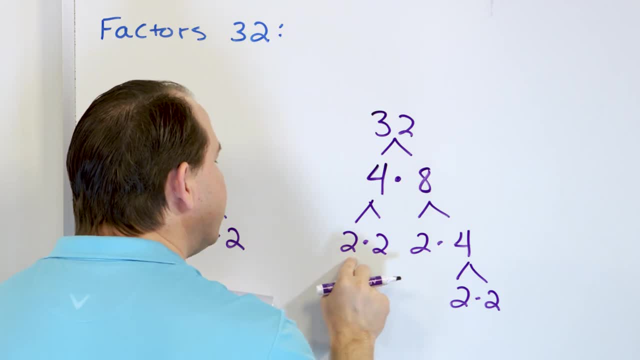 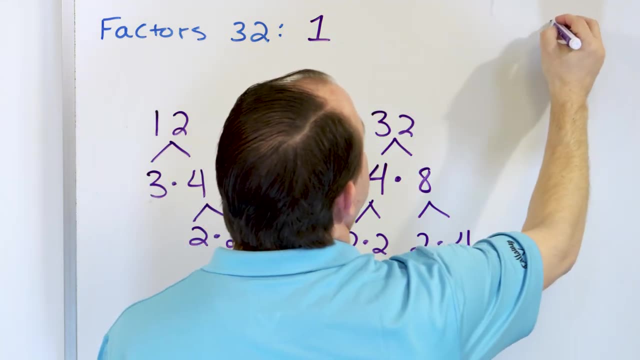 2s, because 2s are prime numbers, I can only break it into 1 times 2,, so I'm just going to stop here. Now I know that the number 1 is a factor, And I also know that the number 32 is also. 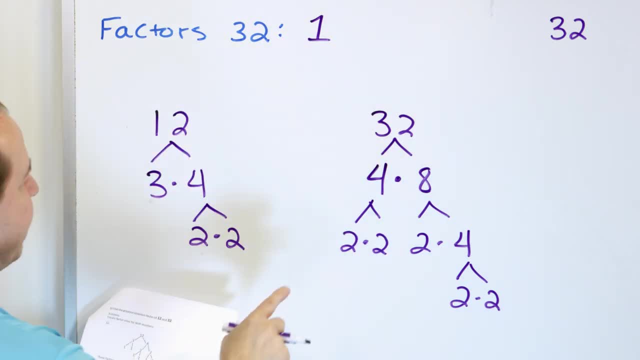 a factor? The number itself. They're always factors. What else do I have in this tree? The number 2, it says is a factor. 4, it says is a factor. What else do we say? It says the number 8 is a factor. I'm going. 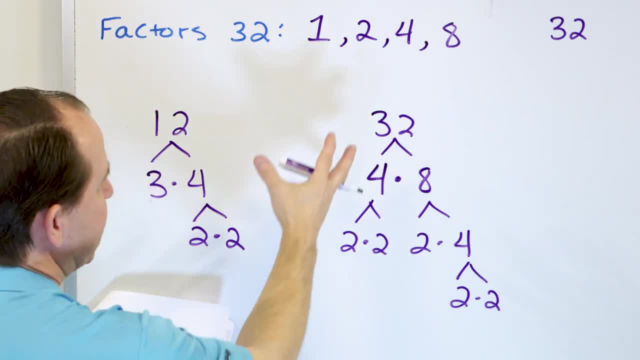 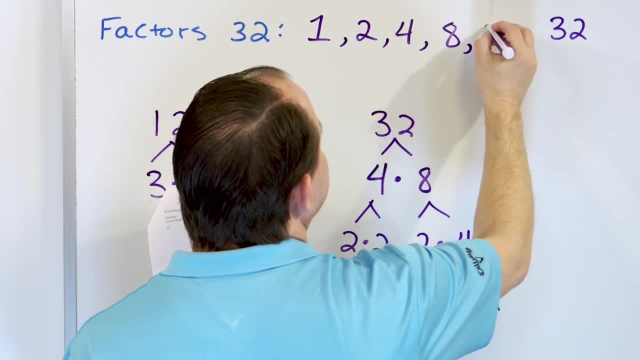 to read that out. So I have 2,, 4, and 8 is also a factor. I've written all the numbers out of the tree. Now let's try to cross. multiply: 8 times 2 is 16.. It says that that's another. 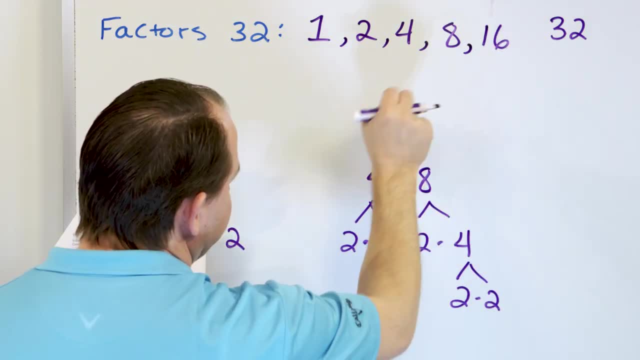 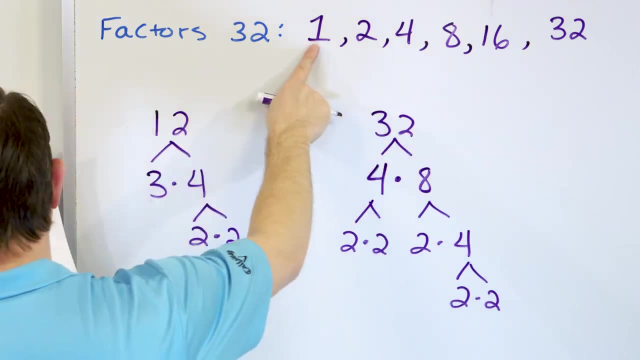 factor Is that all of them 4 times 4 is 16.. Same number 4 times 2 is 8.. That's already in the tree: 8 times 2 is 16.. Yeah, there's no other numbers here, So the factors are: 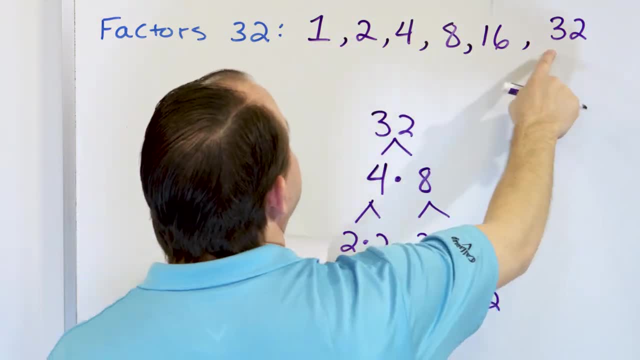 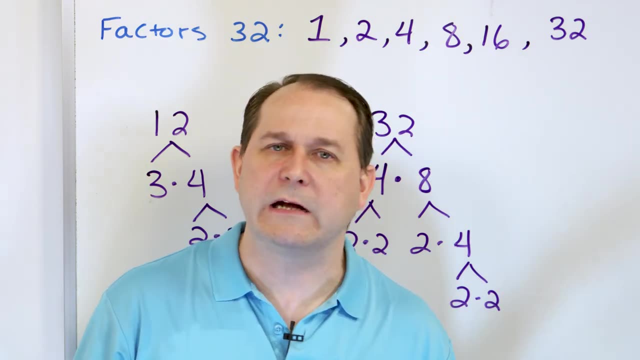 1,, 2,, 4,, 8,, 16, and 32.. The 16 here you might have missed if you didn't use the factor tree, If you were just thinking 3, you might have gotten it, You might not have, I mean. 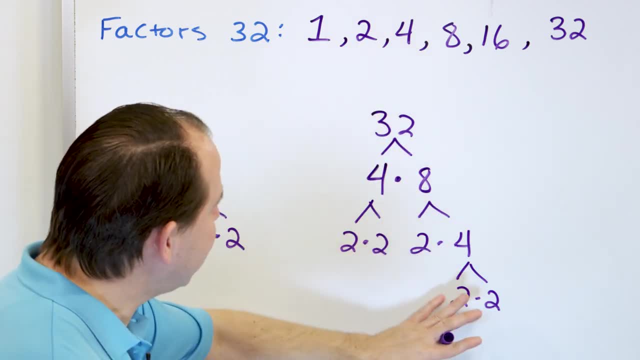 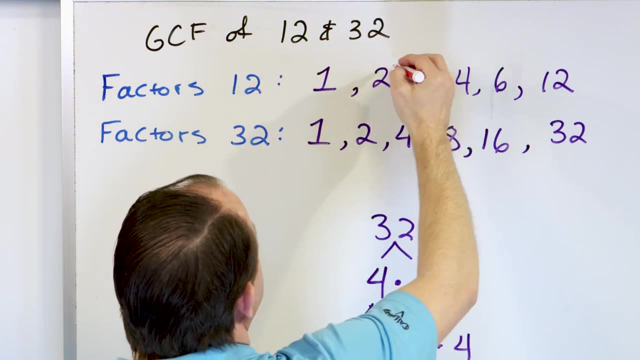 it depends on how you're feeling that day, But write the numbers down out of the tree and then also cross, multiply any branches. So what are the factors in common? 1 is common. 2 is common. 4 is common. What else is common? Nothing else is common above that. So 4 is. 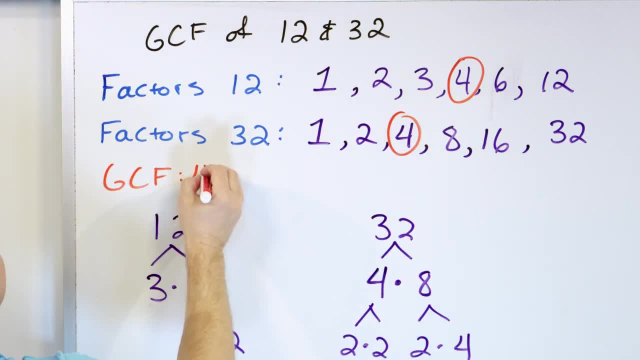 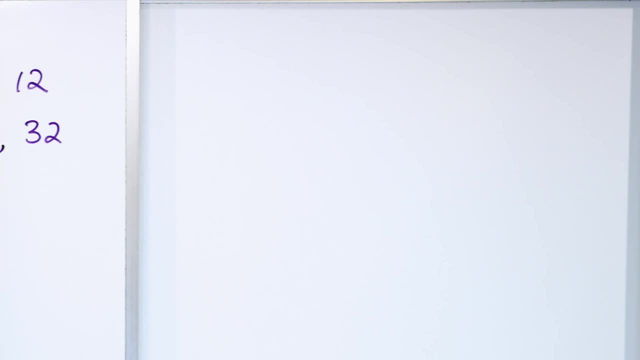 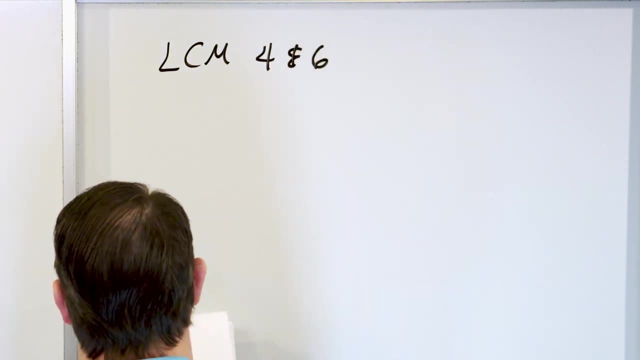 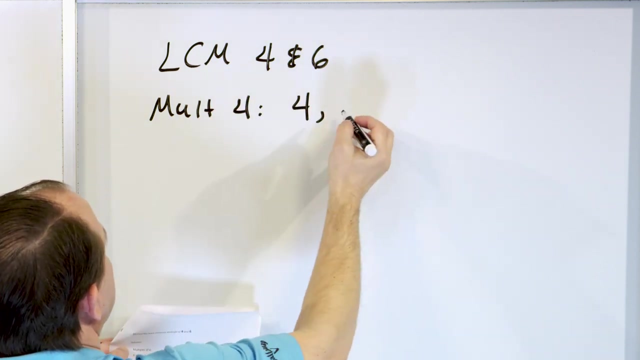 the greatest common factor. 4 is the greatest common factor. The greatest common factor is the number 4.. Alright, here's our very last problem. Let's take a look at the least common multiple of 4 and 6.. So multiples of 4 count by 4s. 4 times 1 is 4.. 4 times 2 is 8.. 4 times 3 is: 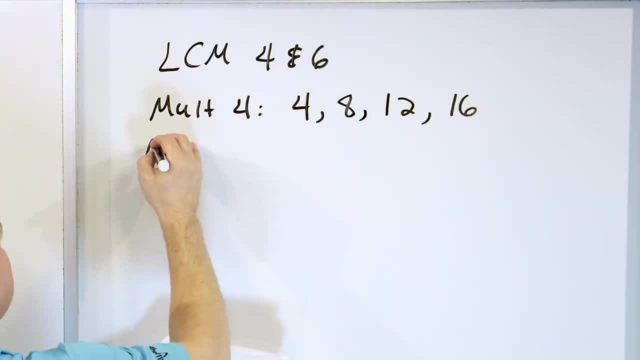 12.. 4 times 4 is 16.. Just stop there. multiples of the number six. I can write the number six correctly. sorry about that. The number six Six times one is six. six times two is 12,. 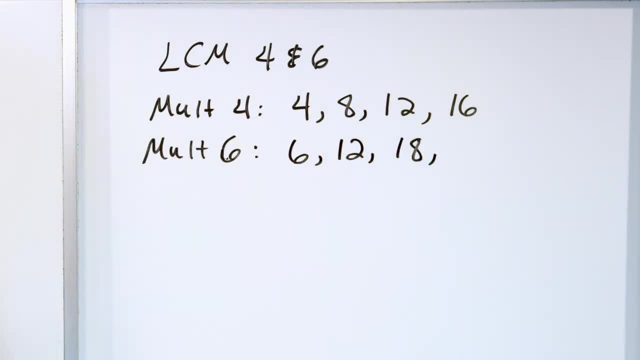 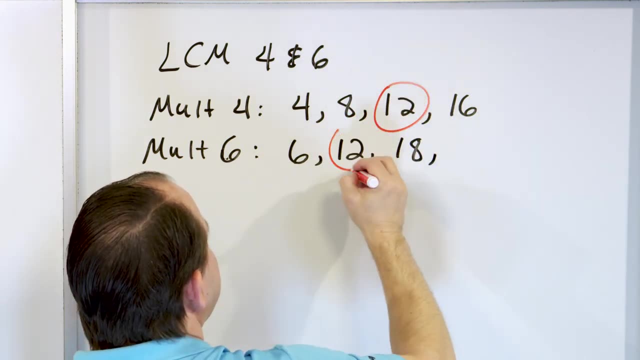 six times three is 18, and you can keep going if you like. What are the commonalities? The only thing I see here is the 12, and of course that's the smallest one that's common to both lists. If I keep going, I'll get more numbers common. 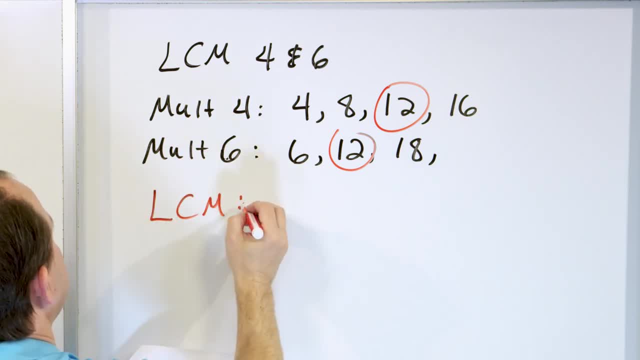 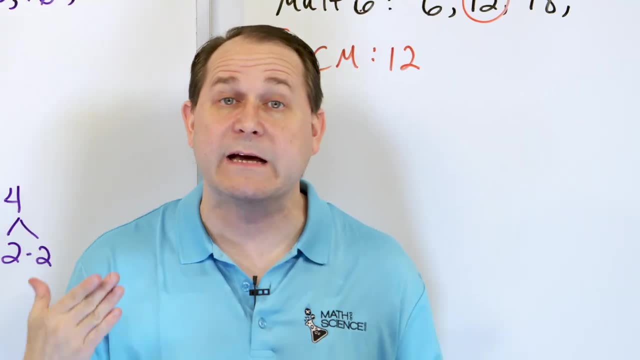 but 12 will be the smallest. Least common multiple is 12.. So I hope, by doing all of these problems, you can see that, even though we have to think about the least common multiple and the greatest common factor, even though we have to work for it, 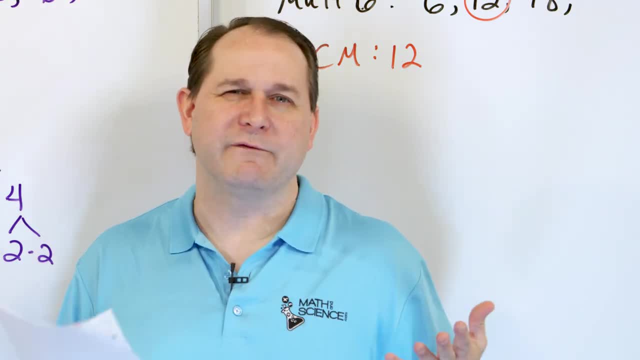 the process is the same for every one of these problems. A lot of people get them confused and mix them together, and I'm really just trying to help you get over that by solving a lot of problems I'd like you to go back through. 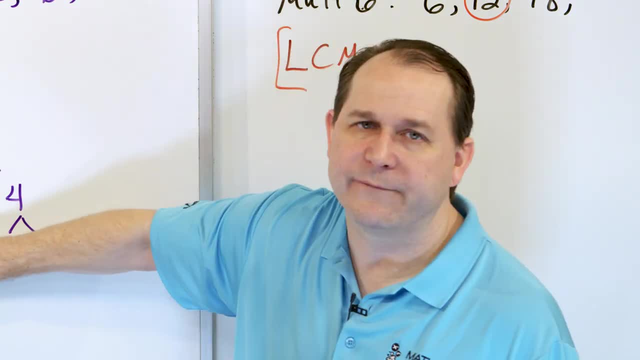 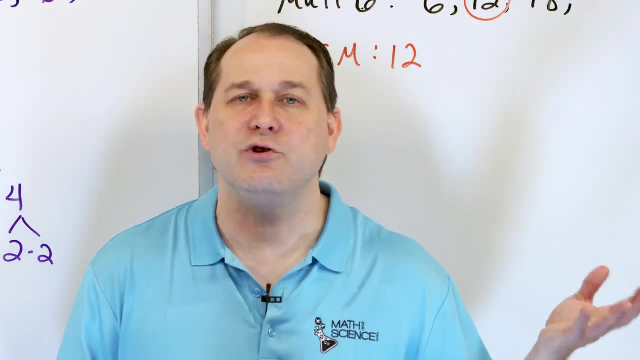 and solve every one of these yourself. and I really do want you to write the factor trees down, because, even though you might not need it for the small numbers, I guarantee you eventually you'll get a problem that you cannot do without a factor tree. 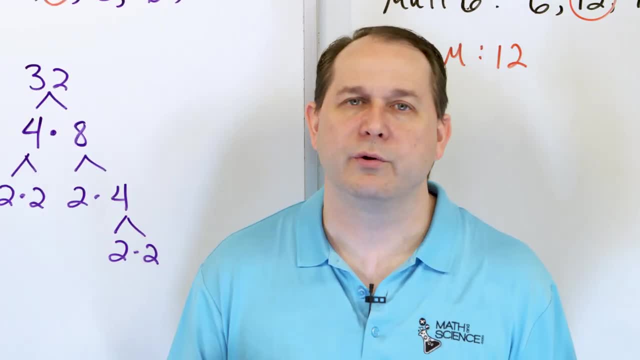 because then the numbers are so big you won't be able to find them all. You'll easily miss a factor. So I'm trying to get you in the habit. plus, they're kind of fun to do, You know. they're like a little drawing. 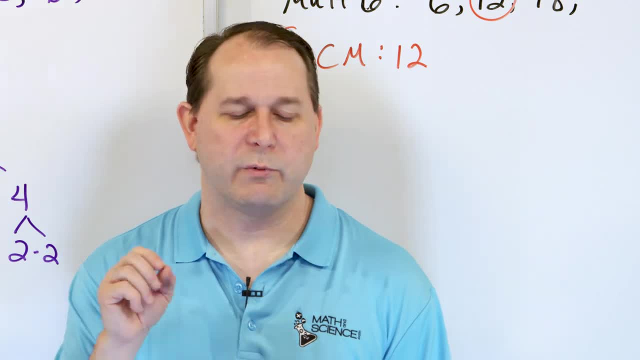 So I would like you to do those. Then follow me on part two, where we will continue skills with factors and multiples.